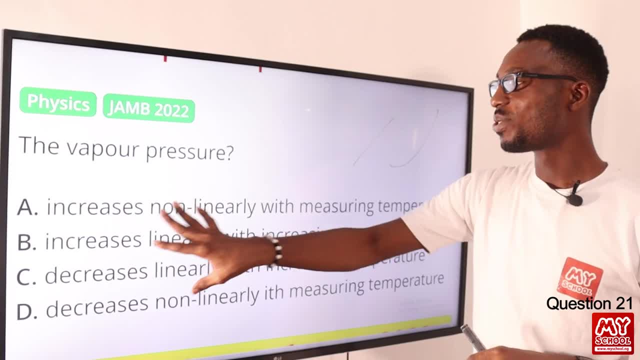 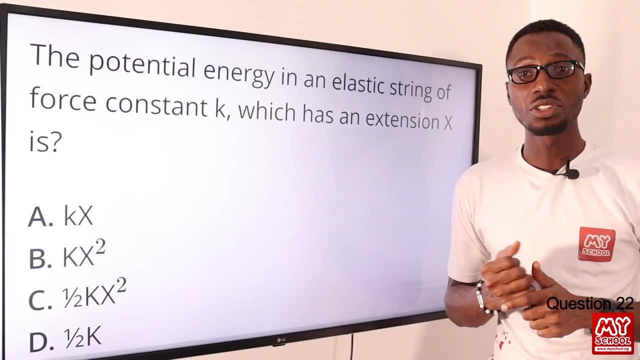 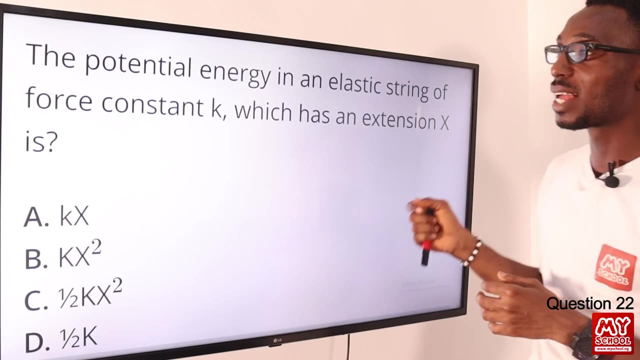 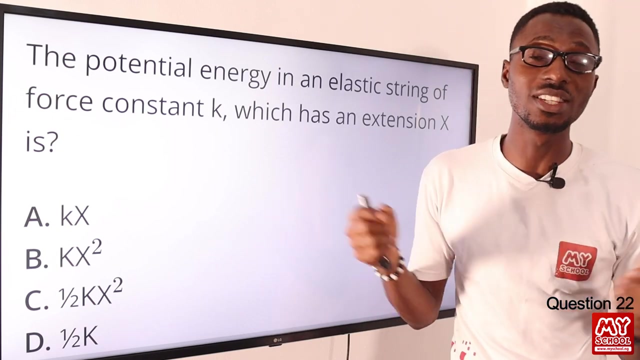 So the correct option here is: vapor pressure increases non-linearly with measuring temperature. So option A is the correct option. Question 22. The potential energy in an elastic string of force, constant K, which has an extension S is what? So, if you recall, you know you are looking at the concepts whereby, provided that the elastic limit is not exceeded, you know the extension produced is directly proportional to the applied force. 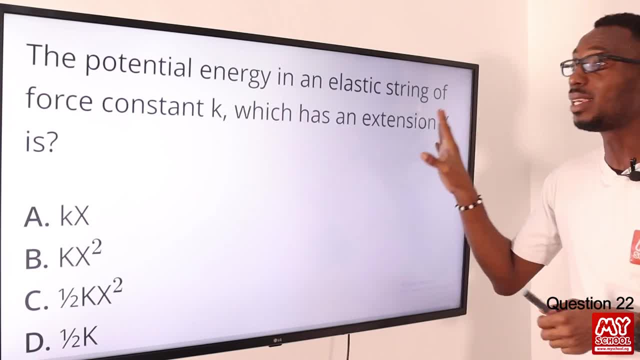 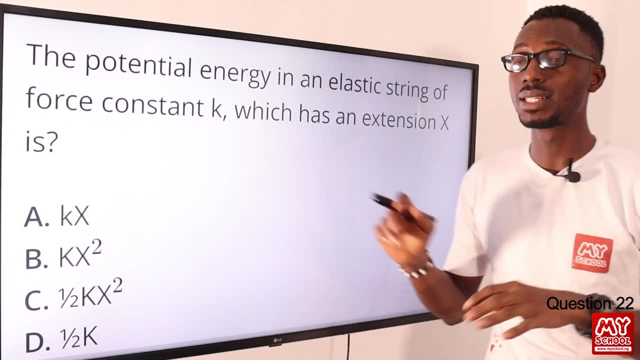 So you are looking at the relationship between the force applied, F and E, the force applied and the extension produced. So, if you now recall that the work done or the energy stored right regarding a particular material, okay, so we are talking about a string here, or a string to put. 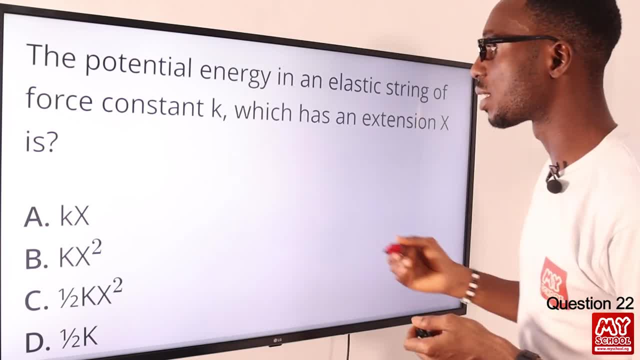 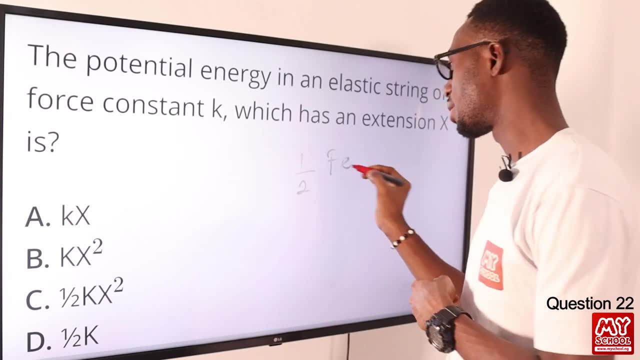 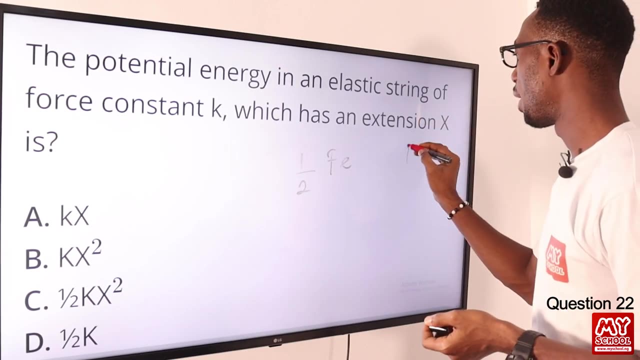 So right. So right now, you want to recall that this expression is actually your average force. you know average force, which is F? right times your extension produced right. So F? E. Recall that your force. okay, remember that we have our F? right equals to K? E. 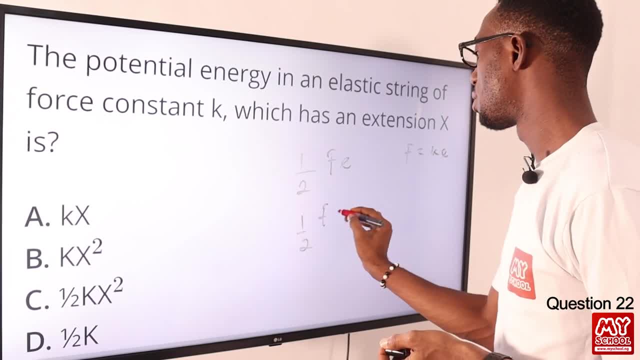 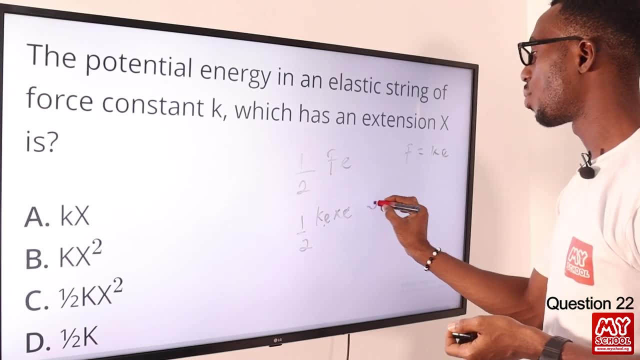 So what do we have? So that would be F right times. okay, F now has been replaced by K E, So I have K E times this E. So what do I have? I have F right, I have K E times E. I have E squared. 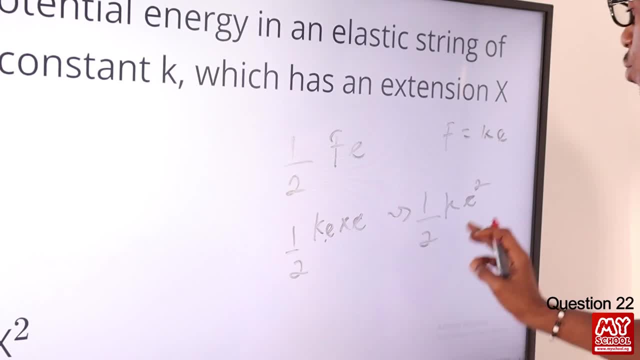 So you just need to recall the formula. then we do an application. So this E is the extension produced and right there it is replaced by, or it is represented by, the letter X. So I have F, K, X. So this is actually gotten from the relationship between the force applied and the extension produced from your Hooke's law. 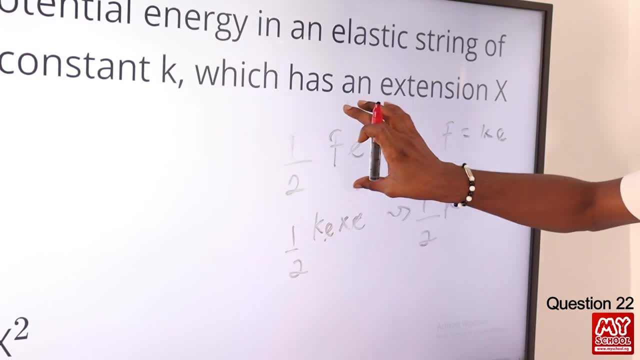 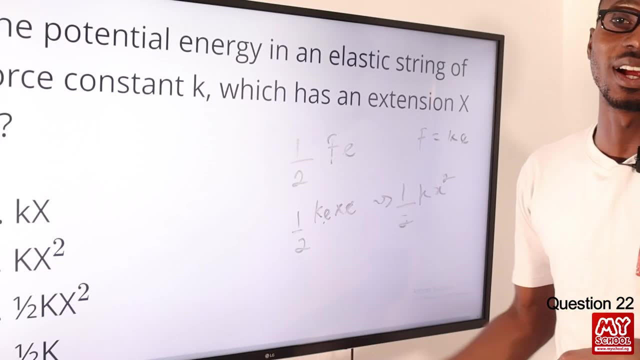 Then if you recall this, then you have your average force applied and extension produced, Then you just replace it By this value, then you get this. So this is just a mathematical expression put together. So the extension E is very represented by X here, not E. 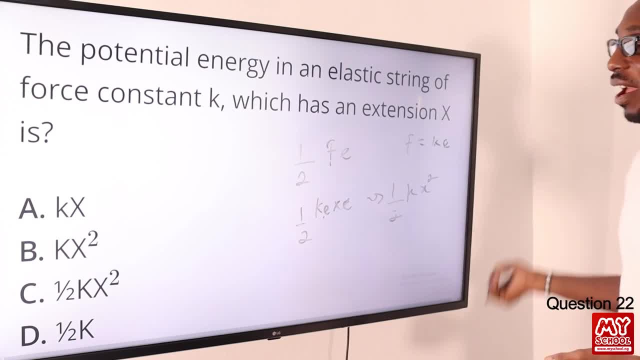 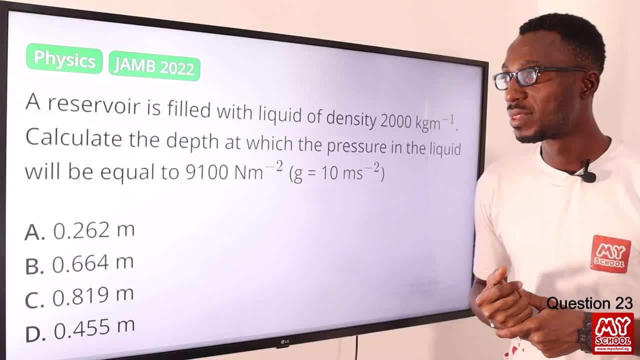 So you see the same thing. So where do we have F, K, X squared? We have that in option C, So option C is the correct option Number 23.. A reservoir is filled with liquid of density 2,000 kilogram per meter. 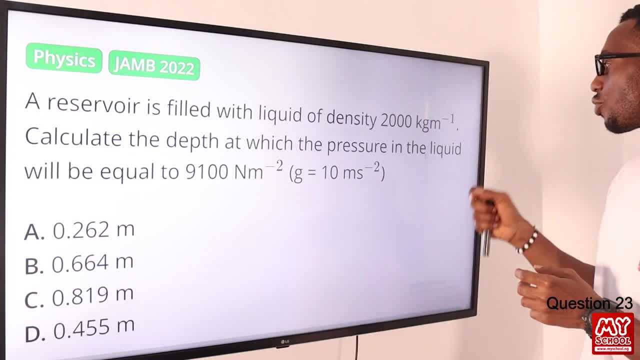 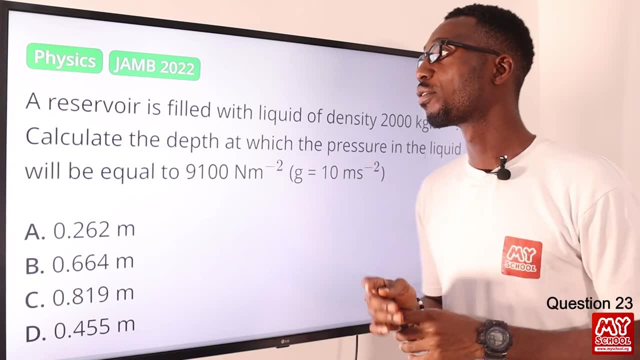 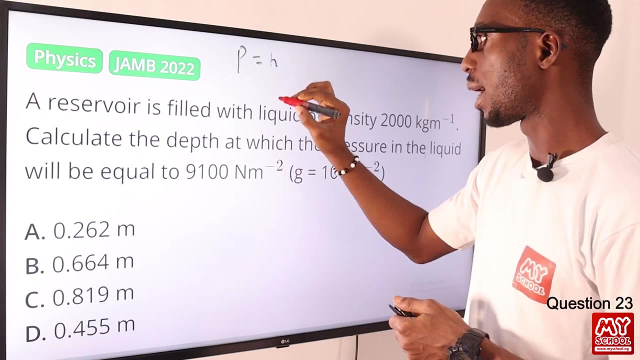 All right. So calculate the depth at which the pressure in the liquid will be equalized. So the pressure is equal to 9,100 Newton per meter squared. So, given that gravity equals to this, So if you want to record relationship between pressure, right? pressure is actually equals to your height or your depth, right? 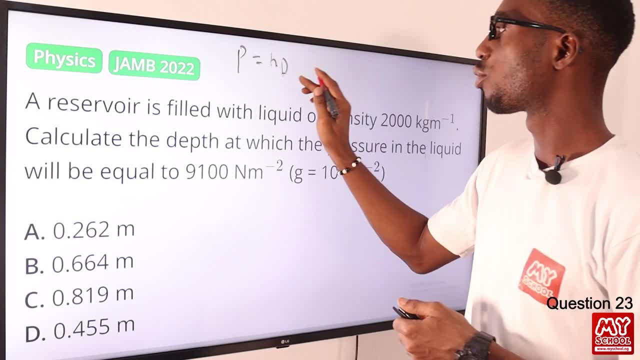 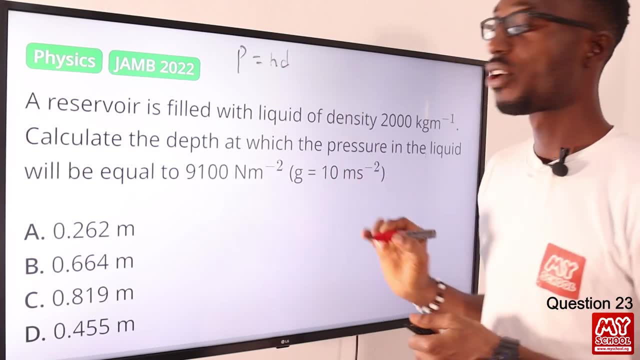 Then times the density. you know certain presentation, we put like this, something like the letter P, but it is not P, So let me just use D to represent density, right here. Okay, And then we have your gravity. So this is a relationship. 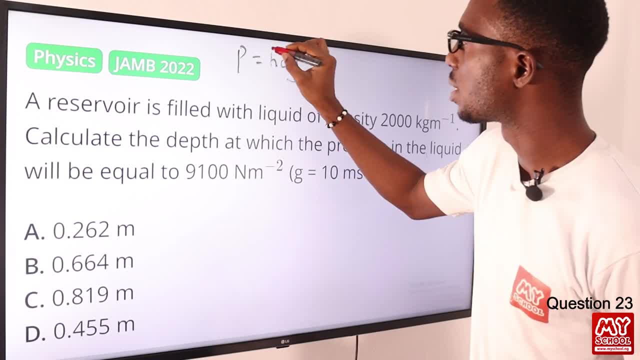 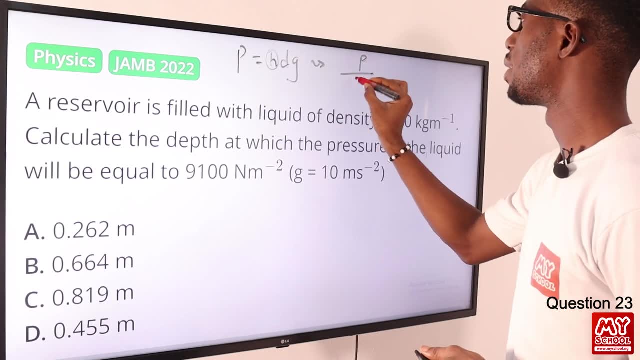 So the question requires that we find the depth, Okay, The height. So this is what we are looking for. So, if we make H the subject of the formula, what are we going to have? We are going to have P over DG equals to H. 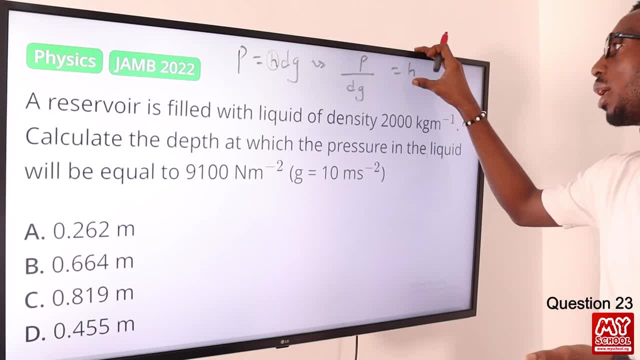 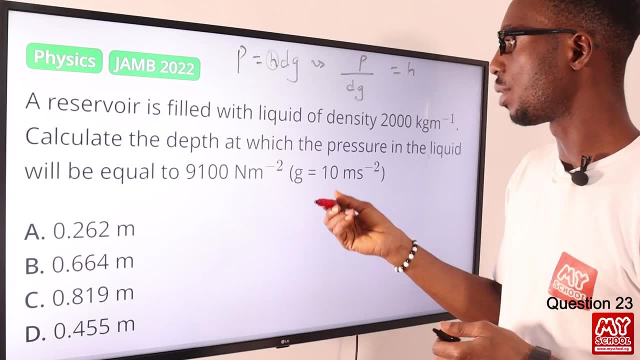 Isn't it? So we are looking for the height or the depth. Okay, So, like I mentioned earlier, some, I think, some articles or presentations or some textbooks will represent your density with something like this: All right, So it's like P, but it's not P. 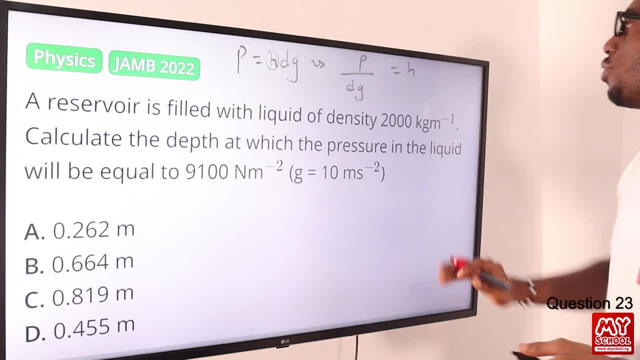 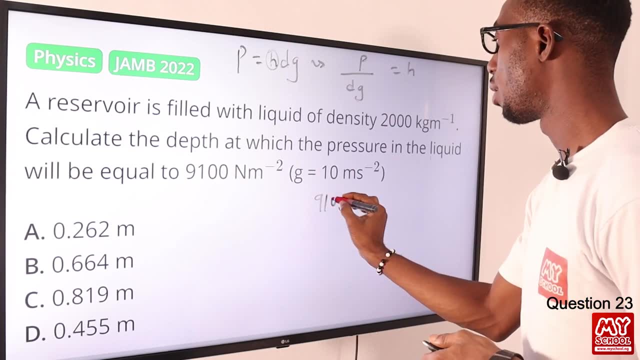 So I don't want us to confuse it with. that's why I'm using this G. So let's put in the supplied value: What is my pressure? The pressure is actually 9,100.. 9,100,, of course. Then what is the density? 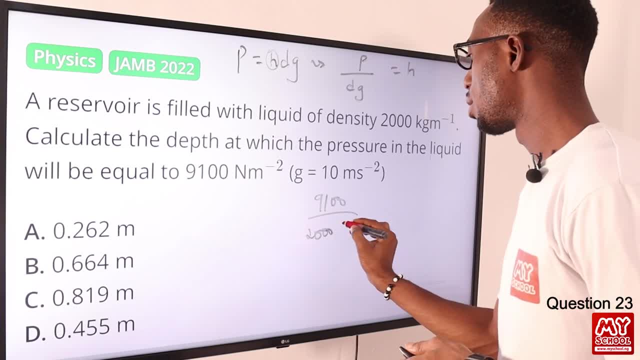 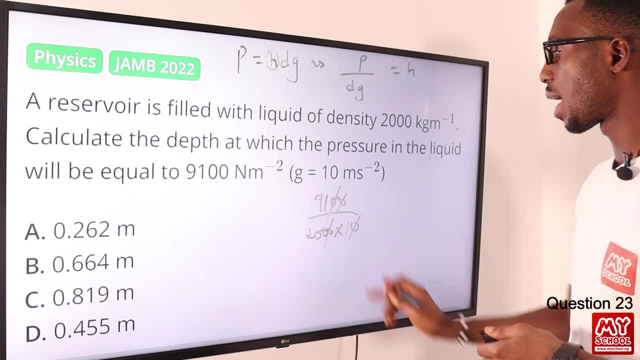 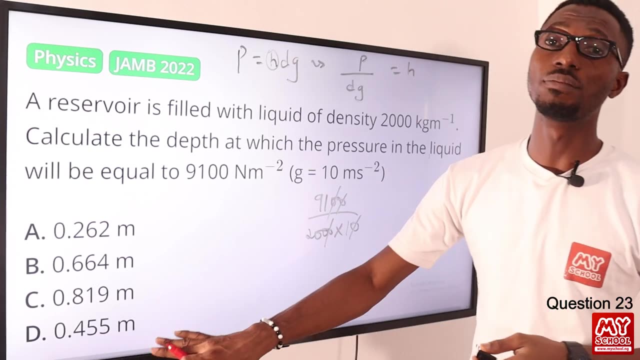 Density is 2,000.. Right Times the gravity, which is G, That's 10.. Right, So it's zero counts to zero, zero counts to zero. So I have 91 over 200.. So 91 divided by 200 will give me 0.455 meters. 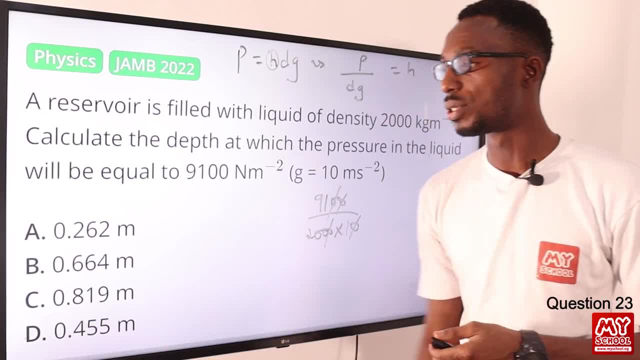 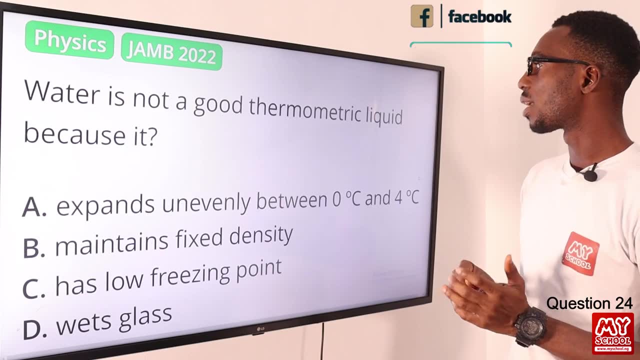 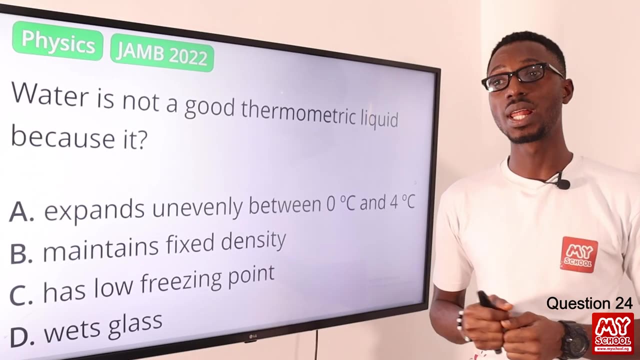 So the depth where we have this experience is found in option D, So option D is the correct option 24.. Water is not a good thermometric liquid because it was So basically, if you look at liquid in glass thermometer, you know we are looking for a liquid that you know its volume responds to temperature. 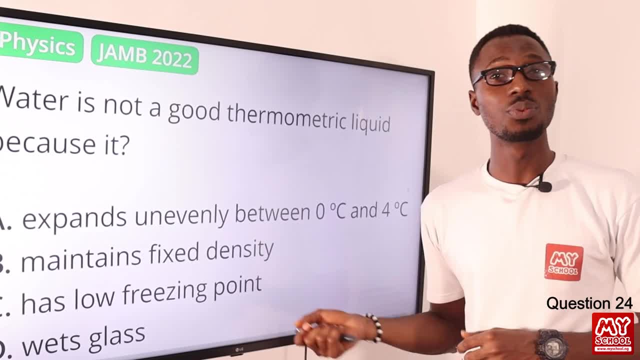 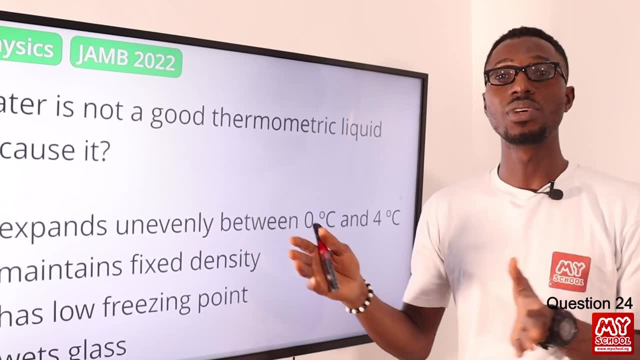 Right So, but that is not really prevalent with water. It's not something we can associate with water, because we have what we call the anomalous behavior. Anomalous behavior of water. You know, between zero degrees Celsius to four degrees Celsius water contracts. 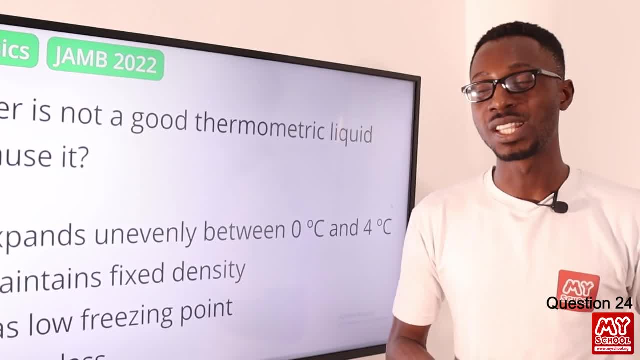 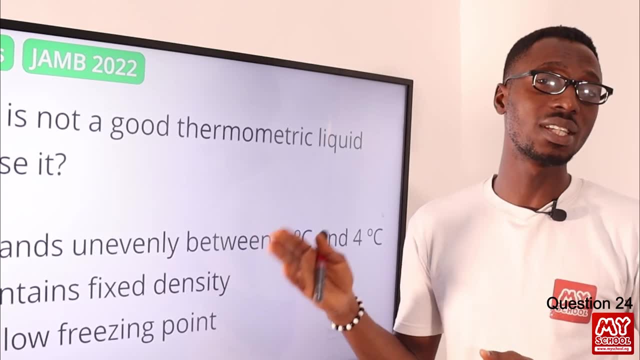 That's why you will now see that high is actually floats on water. So very, very funny behavior regarding water. And again, if you notice that mercury is actually used instead of water, because water will wet the glass- Mercury does not wet glass. 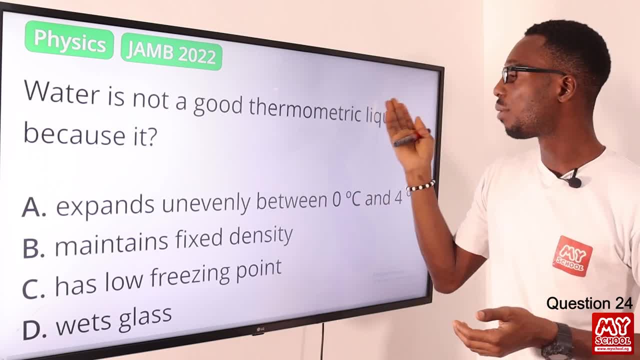 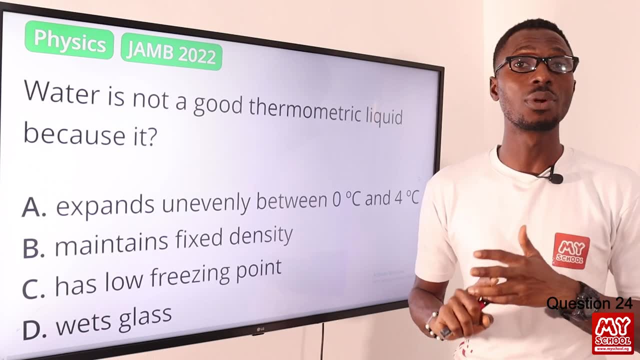 All right. So, when it comes to the context of water not being used as a thermometric liquid, Right, You know you want to look at the fact that it's wet the glass, Its response to temperature, you know it's quite poor. 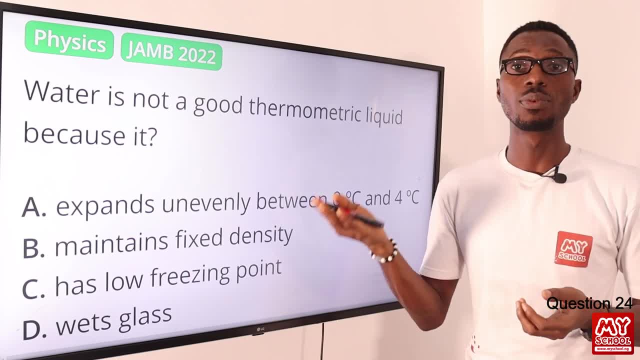 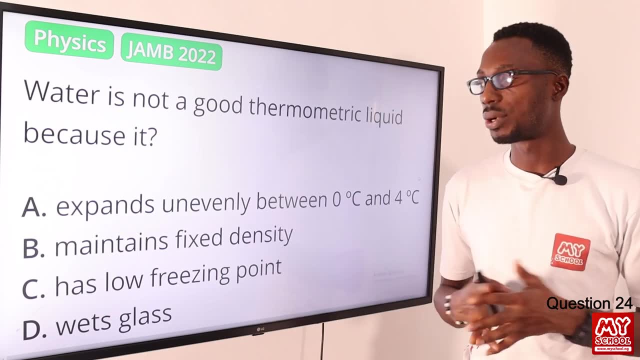 Right In measuring temperature. you know these things have to be very sensitive to temperature change, which we can really find, you know. with water, Then again, we know that water has a high freezing point. you know, in comparison as well. 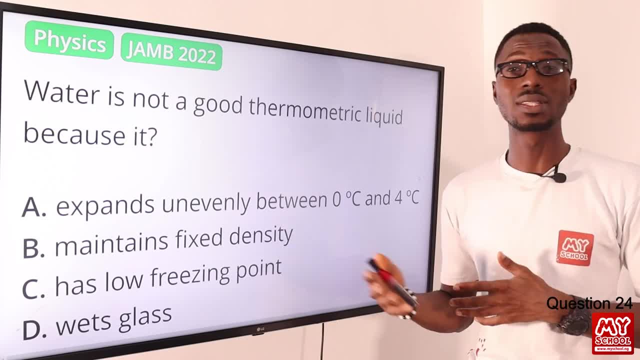 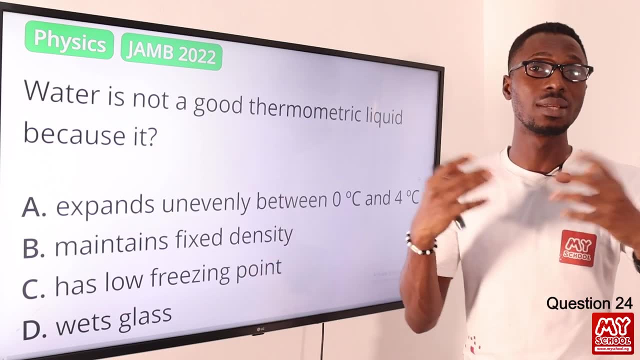 Then we can also tell that water does not maintain a fixed density. You know, for instance, we compare the density of ice to water. You can see that it varies, Even though we are talking about the same substance in different states, Right? 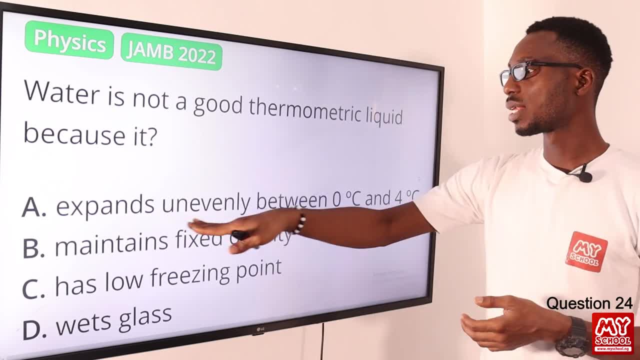 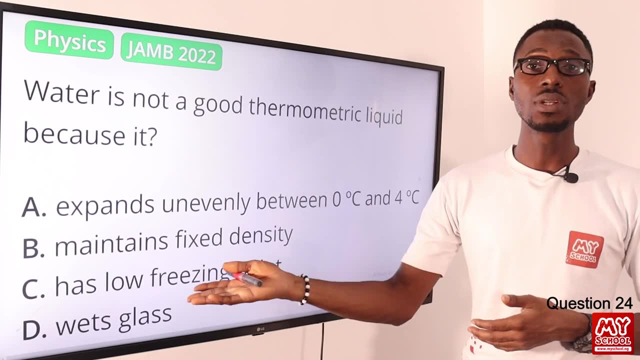 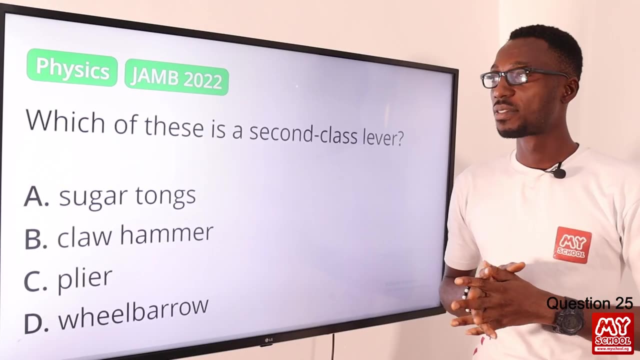 So right. So instead of having expansion it should have contraction. you know its contract between zero and four degrees Celsius, So I feel the most appropriate should be wet glass. option D is most appropriate for this context, Question 25.. Which of these is a second class lever or a second class order or a second order lever? 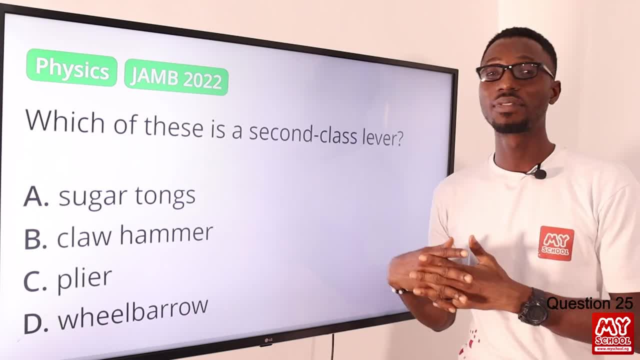 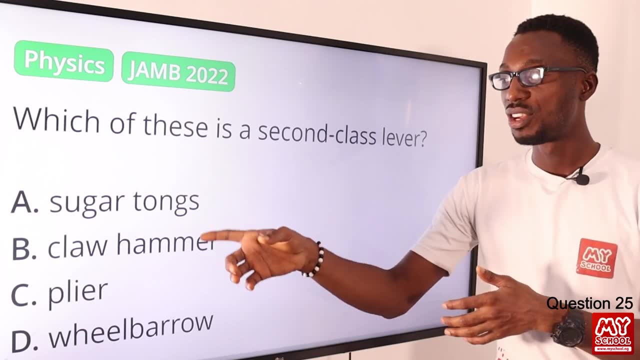 All right, Okay, So you have to first know. okay, the first order, the second order, the third order, All right, So the first order. you are looking at examples: like your claw hammer, you know like your plier, you know like your crowbar. 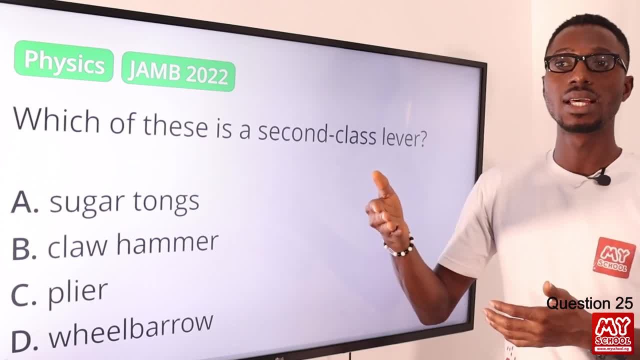 Right. If you look at that arrangement, you realize that the first thing you want to have contact with you know you'll be talking about your load. For instance, look at your plier. you know you have your load right here. 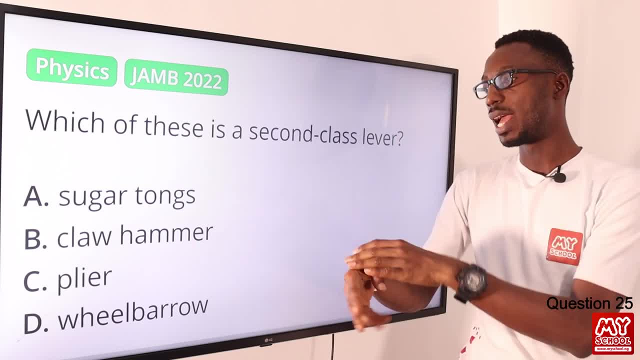 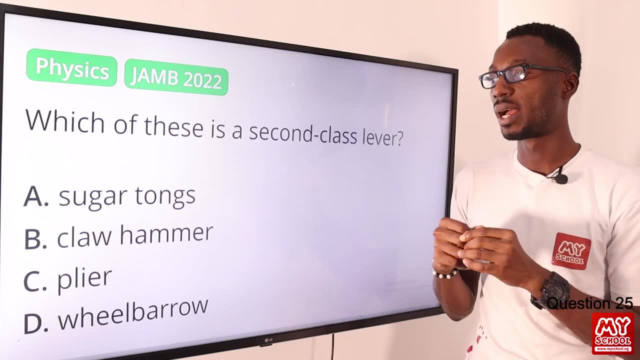 Right. Then you now talk about your fulcrum, Then the effort. This is where we are applying the effort, you know, to actually grip whatever material that has been stuck in the mouth of the plier Right. So these are first class. 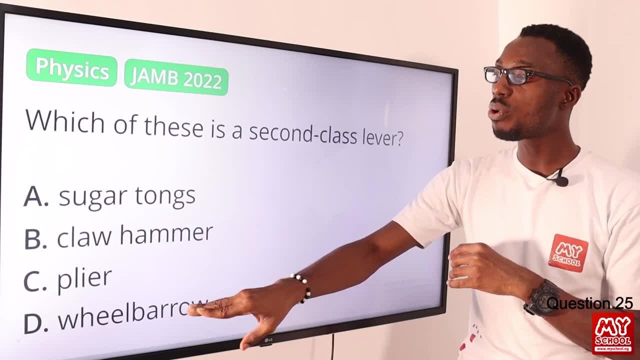 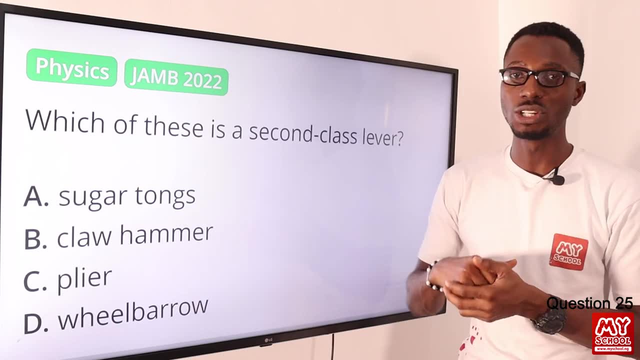 This is third class, All right. So this is actually an example of a second class lever. So another example is your nutcracker. you know where you have the load in the middle. So the correct option is option D, four wheel barrel. 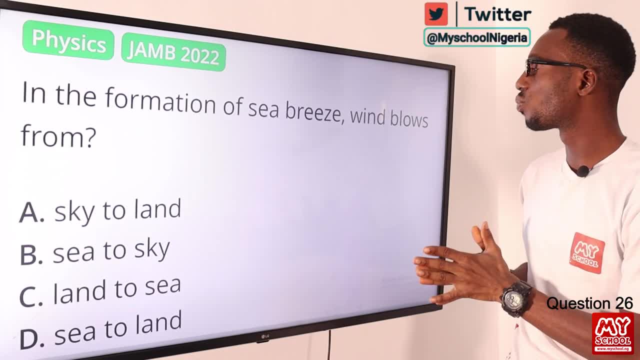 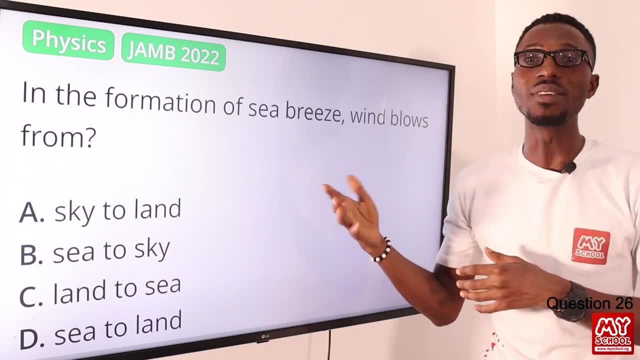 Question 26.. In the formation of sea breeze, wind blows from where. All right. So when you look at the sea breeze, the land breeze, just as the name implies, you know. sea breeze, That is the wind coming from the sea to the land. 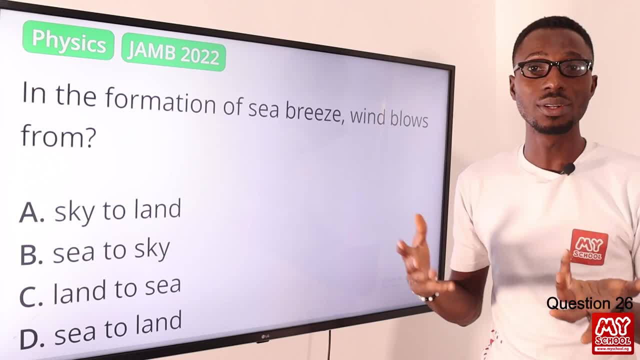 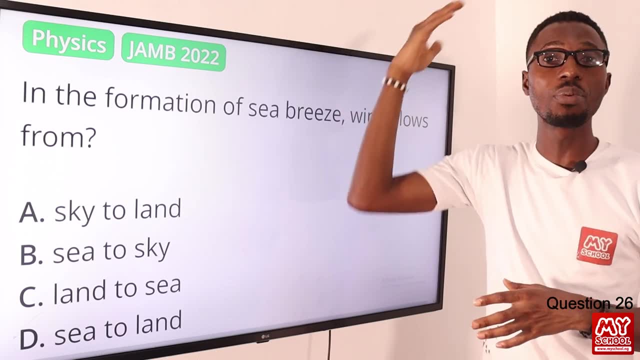 Because during the day you realize that the ground is being heated up Right, So the air there is hot, So it rises Of course. So you now see that the cool breeze you know from the sea will replace what you have already. 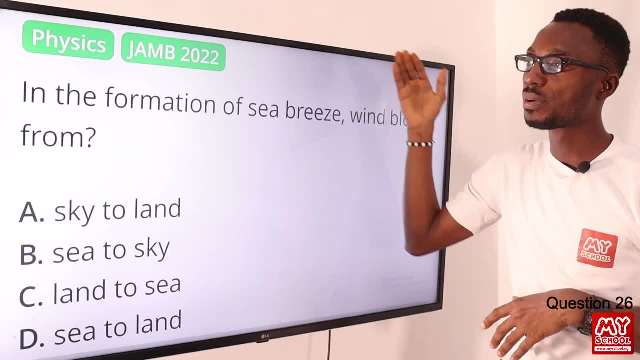 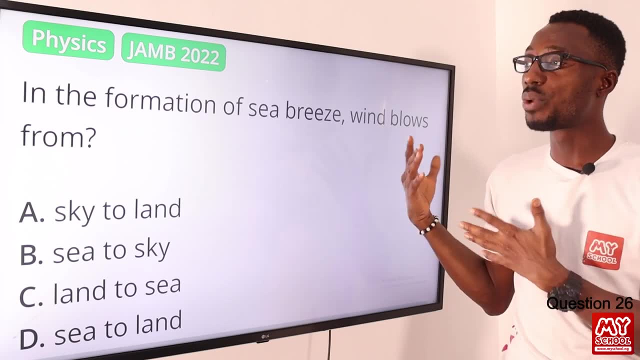 on land, So that one has already gone up Right. Then the cool breeze from the sea comes to replace. Then at night, you know, the reverse happens. So definitely the formation of sea breeze is when wind blows from the sea to the land. 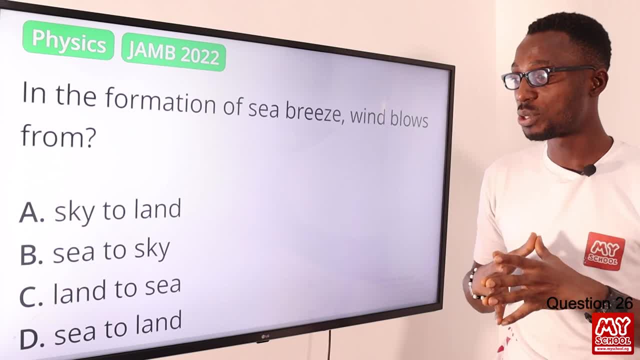 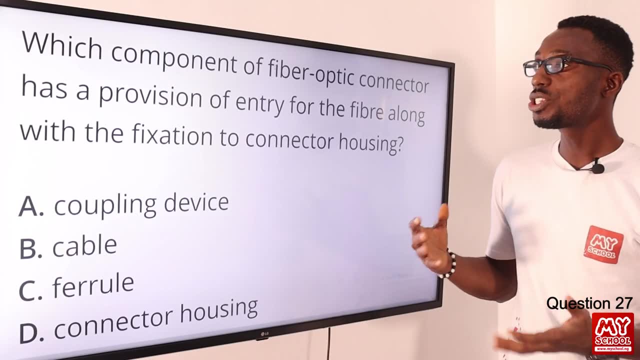 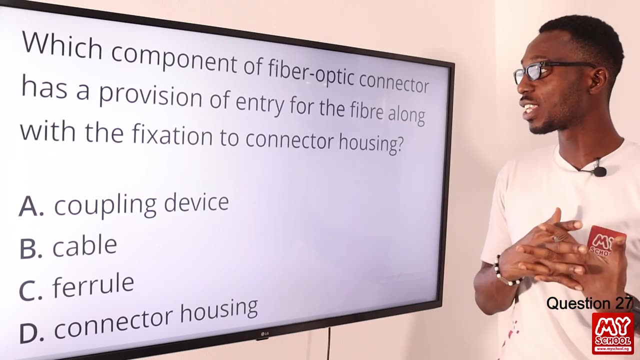 All right. So where do we have the correct option? We have that loaded in option D, So option D is the correct option, Number 27.. Which component of fiber optic connector has a provision of entry for the fiber, along with the position to connector housing? 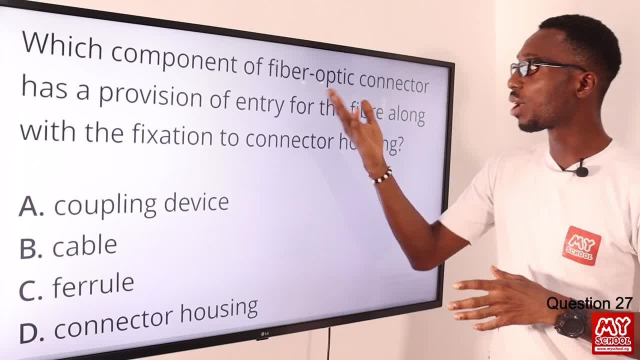 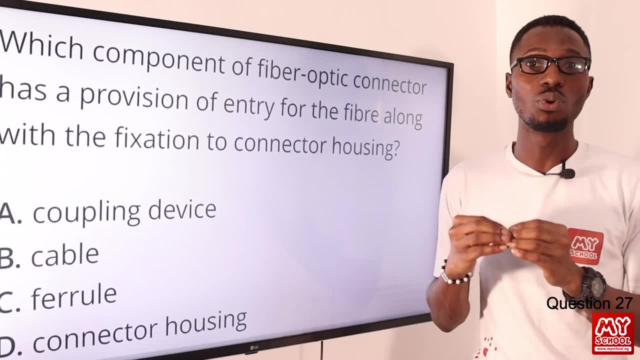 So basically, we are looking at a coupling device, or you can refer to it as a fiber optic coupler. All right, So what this does is that it's just an optical device. You know, Probably you want to merge a single. you want to merge one or two inputs into a single. 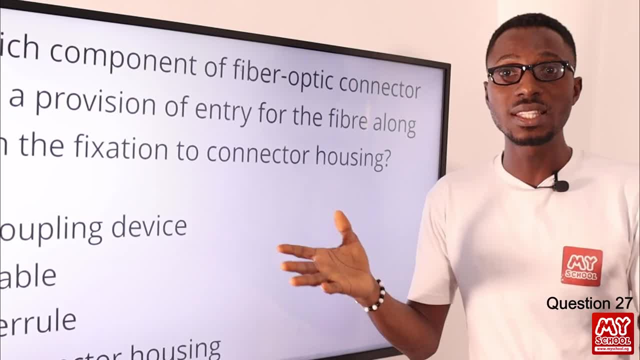 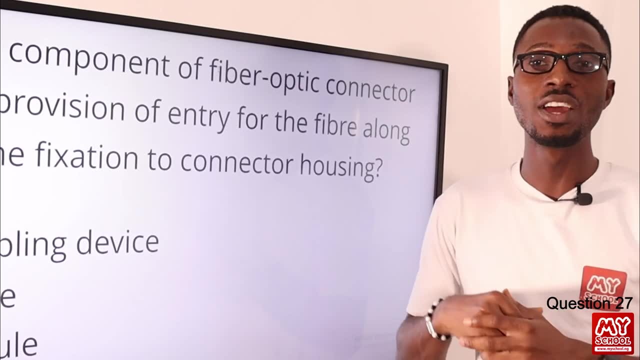 output, or you decided to split a single input into two or more outputs. So that is where the coupling device comes in. So sometimes, based on the functionality, you can refer to it as you know: a combiner or a splitter. All right. 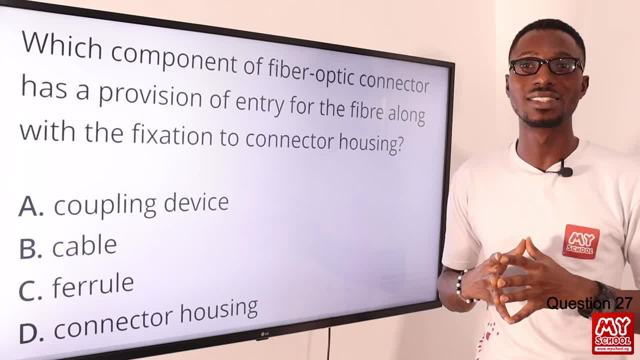 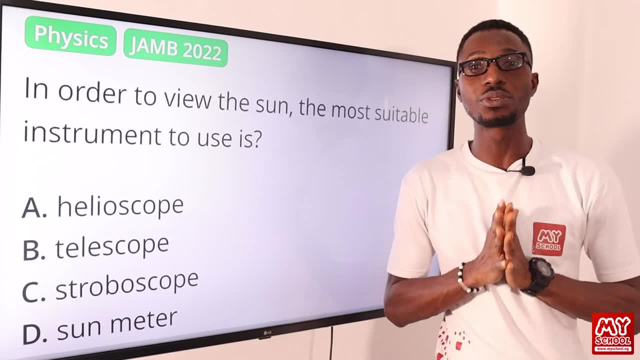 So, basically, the correct option is option A for coupling devices. Don't forget that. Now it's very important that you have a JamCBT simulated experience. All you just need to do is to click on the link in the description below. This is going to get you to the MySchool website. 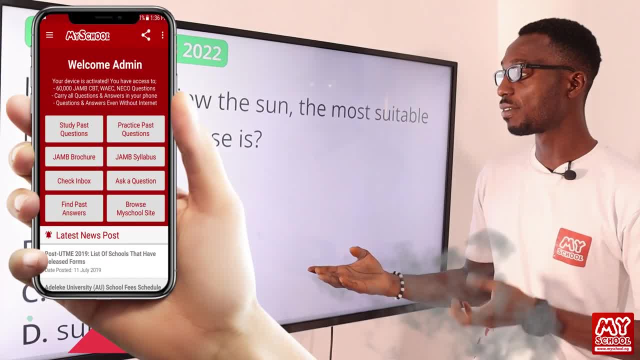 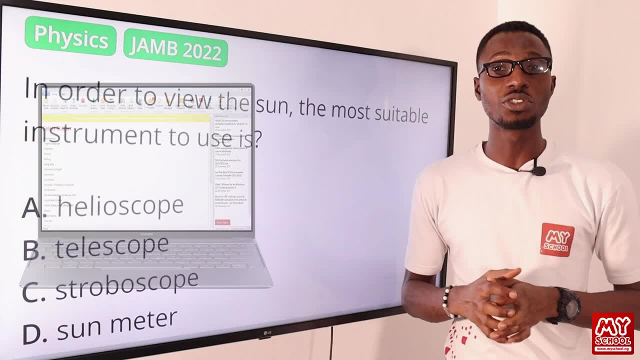 So right here you get to download the MySchool mobile app for your Android devices, or you can go for the MySchool software for your computers and your laptops. So join me as I tackle question 28.. In order to view the sun, the most suitable instrument to use is what? 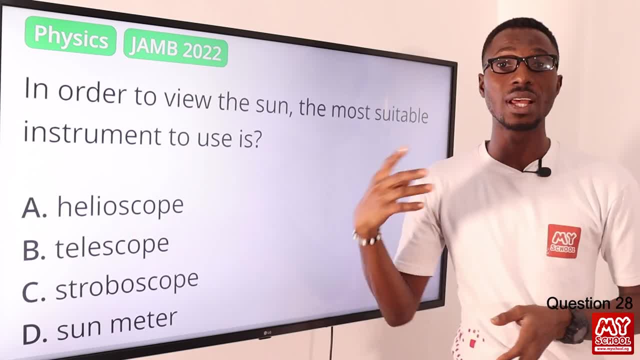 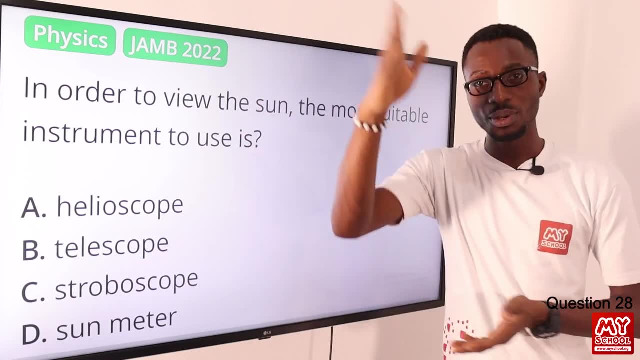 So the most suitable is, of course, the Helioscope. You know You want to observe the sun and the sunspot. This is what you use. Telescope: you know you want to view distant objects, right? You know in the space, outer space, right? 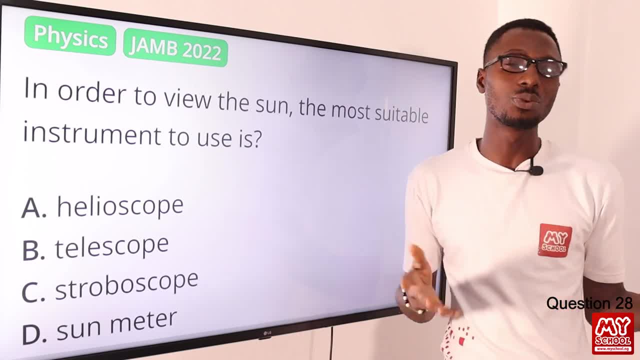 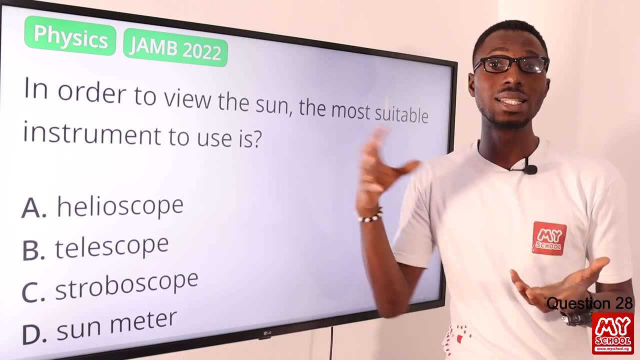 So the stroboscope? you are talking about rotating speed, right Then the sunmeter. you know, or sometimes it's called the solar meter- You know you actually want to measure the intensity of sunlight. you know that falls on a particular surface. 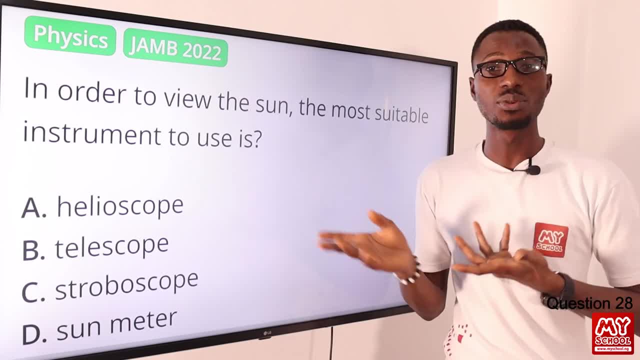 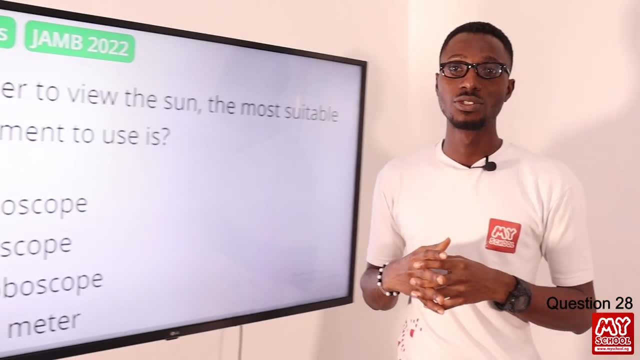 Probably in the context of you know, the solar power regarding household usage and the like. So the correct option is option A for the Helioscope. Do not forget that you have to hit that like button, Click on the subscribe button and always tap on bell notification for you to get alerts. 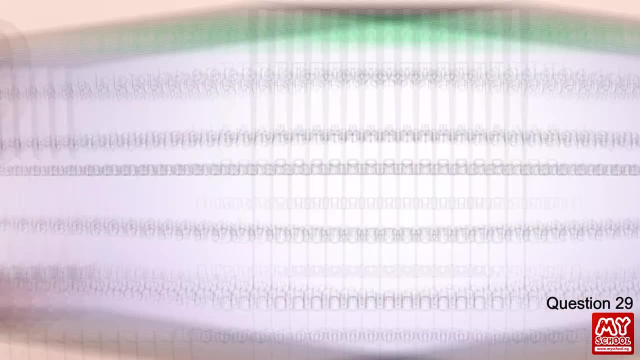 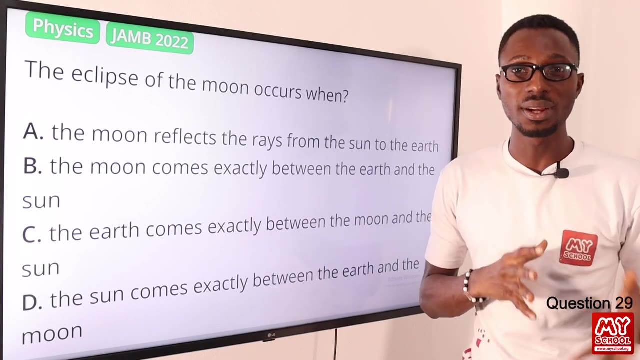 Immediately we upload the next video content: Question 29.. The eclipse of the moon occurs when: All right, So eclipse of the moon is when the Earth comes between the sun and the moon, All right, The eclipse of the sun is when the moon comes between the sun and the moon. 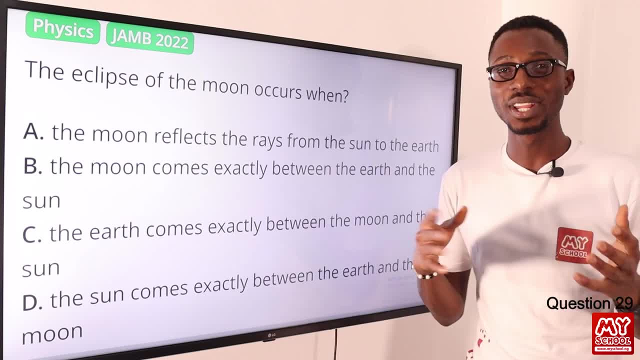 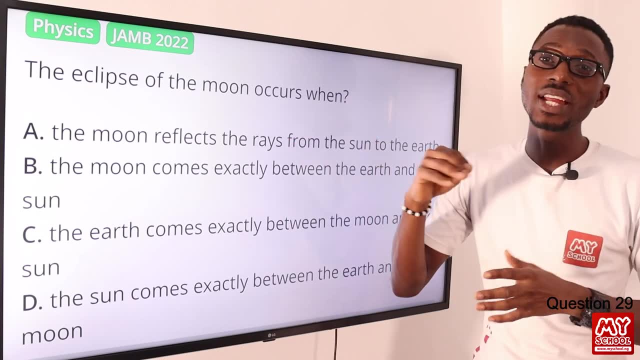 All right between the Sun and the Earth. So don't get it mixed up. You just need to practice, All right. So what do we have of the right combination? You know, the eclipse of the moon occurs when the Earth comes between the Sun and the Moon. So where do we have that? We have that in option C, The 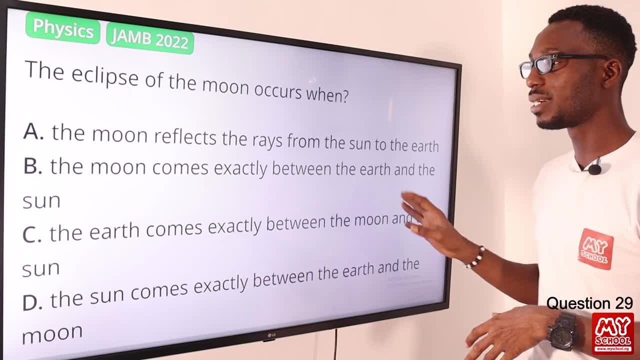 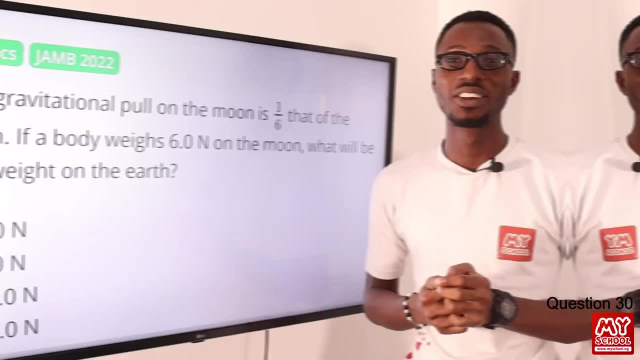 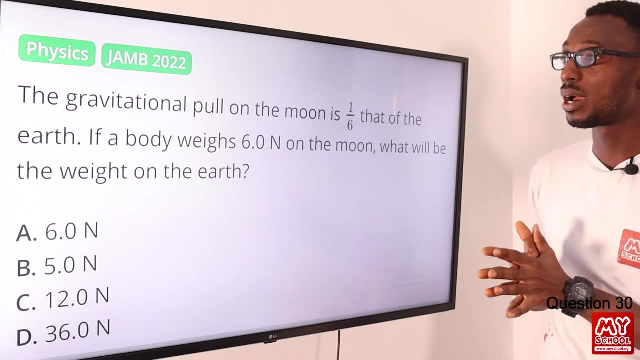 Earth comes exactly between the Moon and the Sun. So you can have a form of eclipse, either partial or full. So the correct option is option C. Question 30. The gravitational pull on the Moon is 1 sixth that of the Earth. It's 1 over 6 of that of the Earth. So if your body weighs 6, 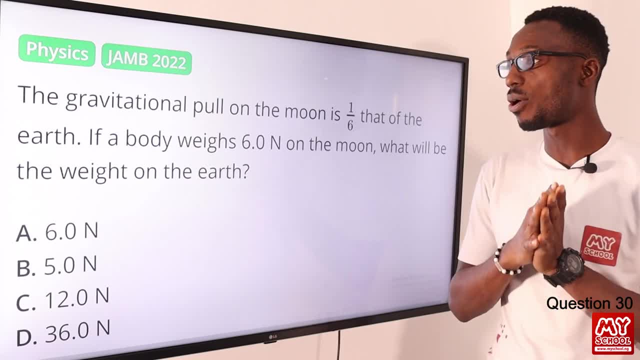 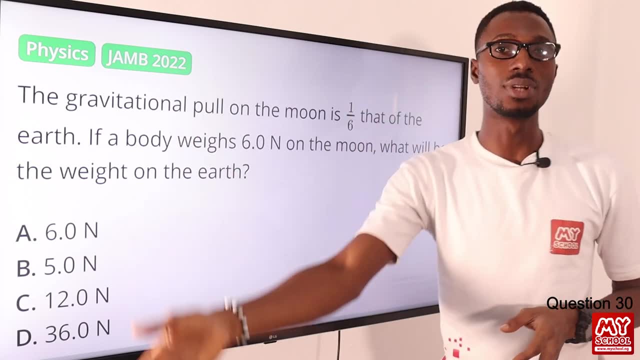 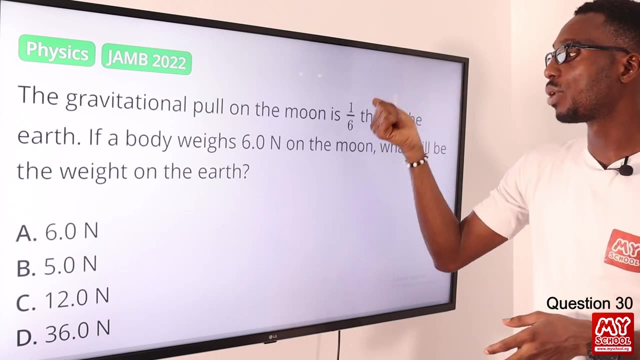 newtons on the Moon, what would be the weight on the Earth? So, basically, if the person is weighing 6 newtons on the Moon, then that means it is times 6 on Earth, right? Imagine if the person is weighing 30 on Earth. So what would be the weight on the Moon? That would be 1 over 6 by 30. So if 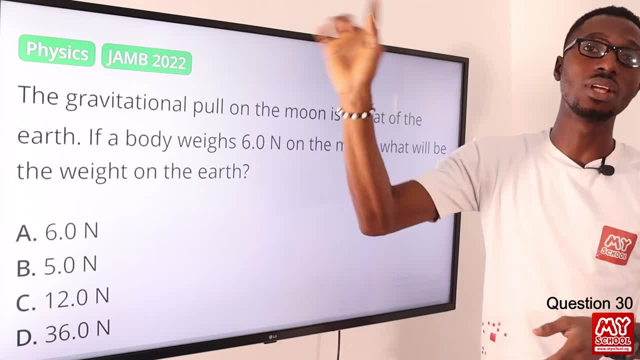 the person now is weighing 6 newtons on the Moon and is now coming to the Earth. it's just weight times 6, you know of whatever. So that would be 6 newtons times 6. That is 36.. So 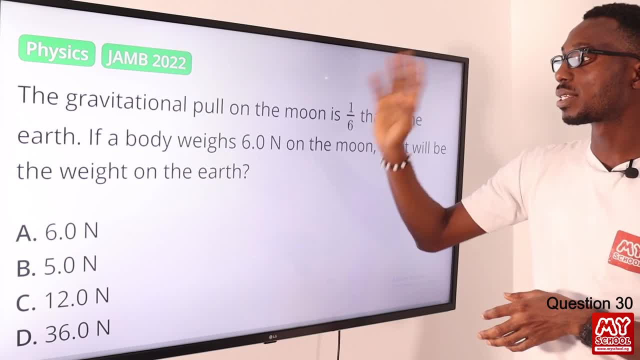 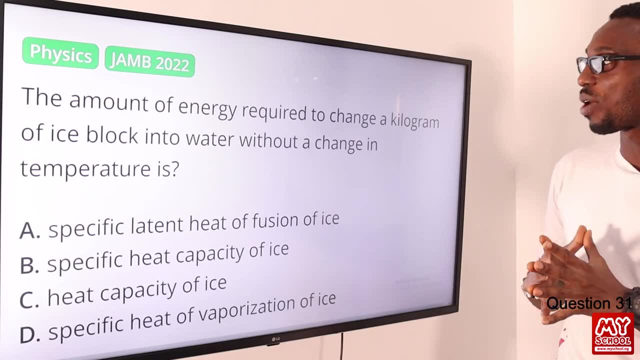 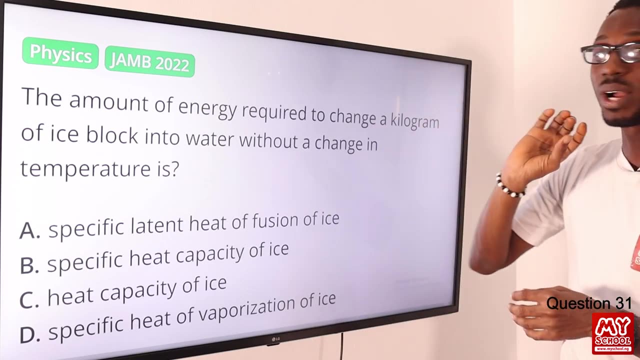 the person will weigh 36 newtons on Earth and weigh 6 newtons on the Moon, So the correct option is D 31.. The amount of energy required to change a kilogram of ice block into water without a change in temperature is what? So look at the keywords that we have here. A change in kilogram. 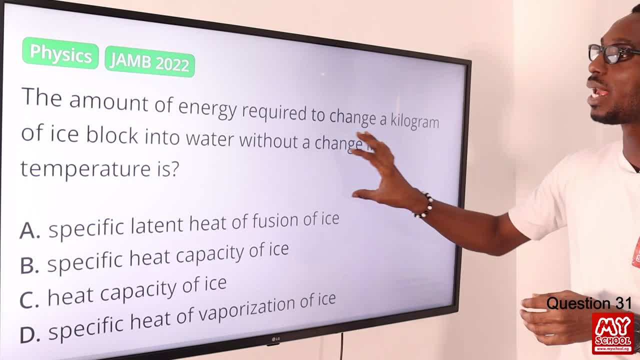 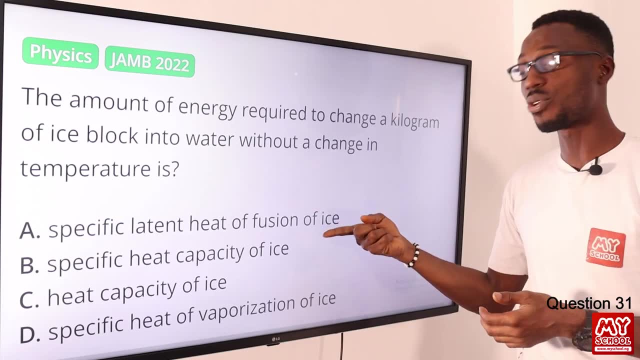 you know, we are talking about a unit mass, right? Then also without a change in temperature, right? So this is where specific latent heat or fusion comes in, And in this context, we're talking about ice, right? So, basically, if you look at the concepts of specific latent heat or 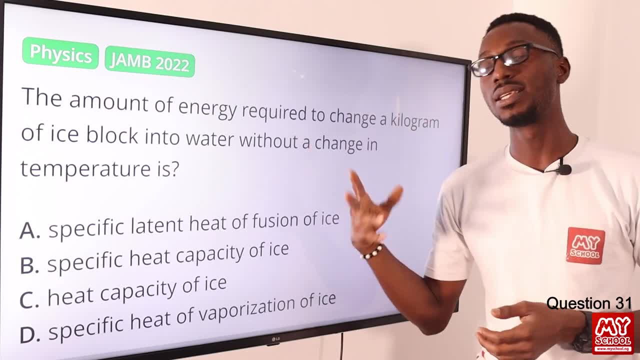 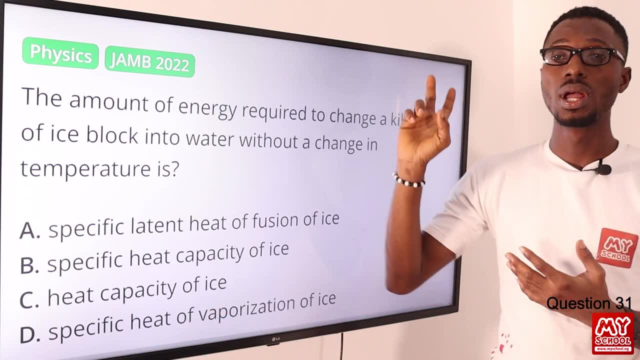 fusion, you know you're actually changing a unit mass of a solid right into liquid right without a change in temperature. For vaporization: you know specific latent heat or vaporization. you know. for vaporization, you're looking at change, you know, from liquid into vapor. 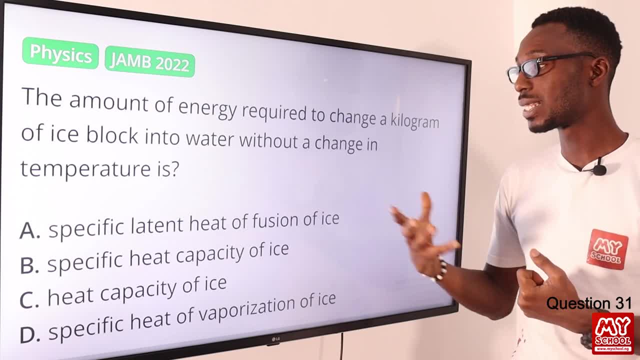 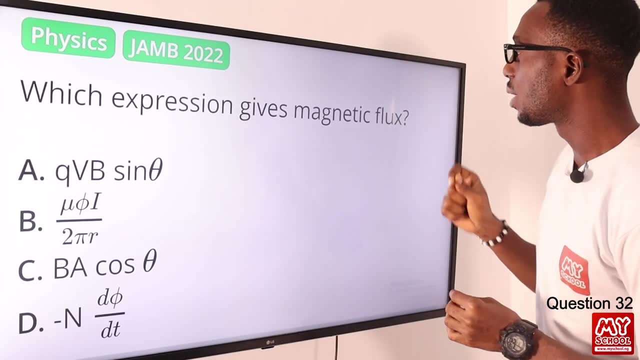 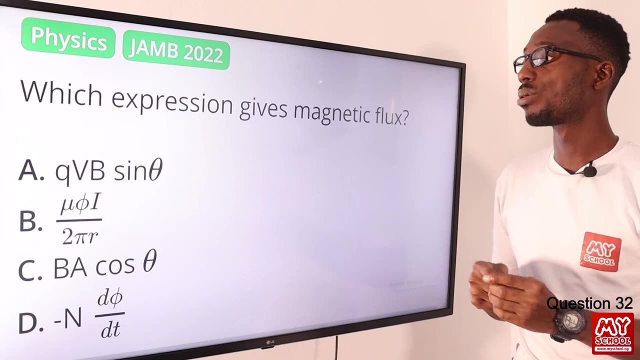 right. So the correct option is option A: Specific latent heat or fusion of ice. So A is good to go. 32. Which expression gives magnetic flux? So when you talk about magnetic flux, you know the units. you can use Weber, right? So we? 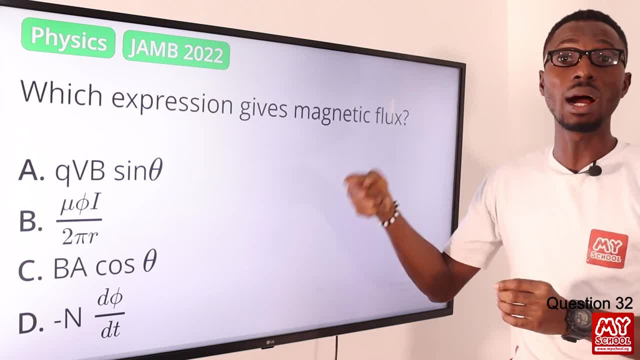 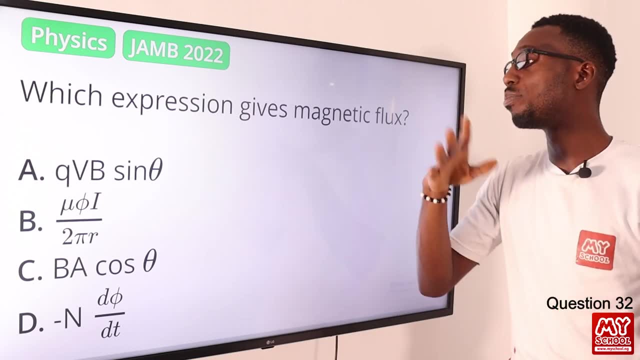 are looking at that rapport between the amount you know of magnetic field, right, which travels, you know, perpendicular to the area. okay, Basically, that's just so. we're looking at the relation between magnetic field and area, all right. 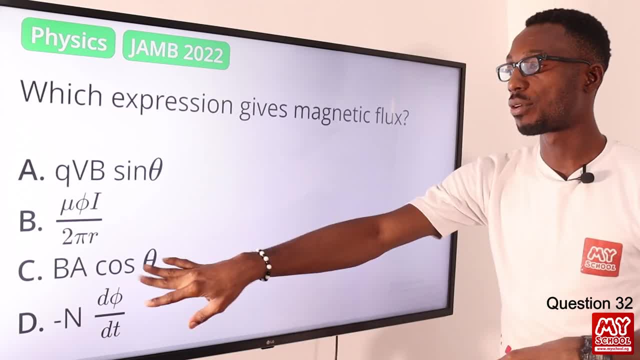 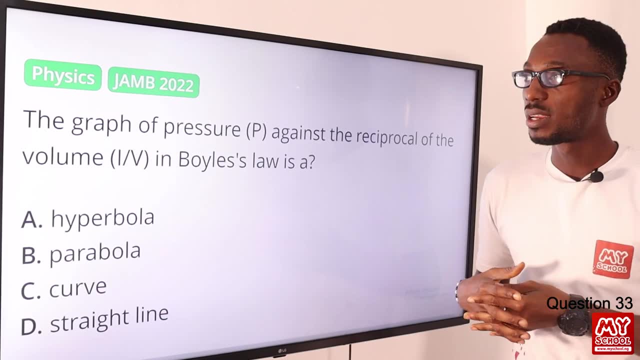 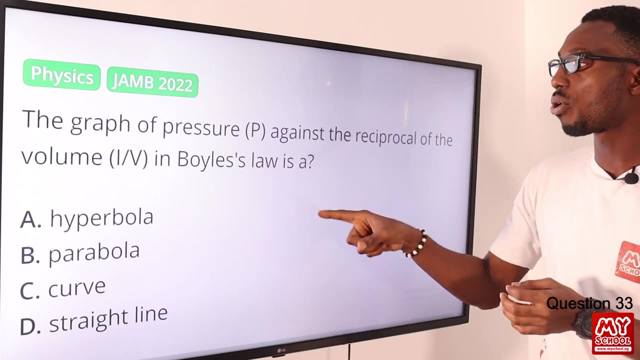 B stands for the magnetic field, then A the area. then we have cos theta. So the correct expression here is actually BA cos theta in option C, Number 33.. The graph of pressure P against the reciprocal of the volume, right inverse of volume in the Boyle's law is a. what? 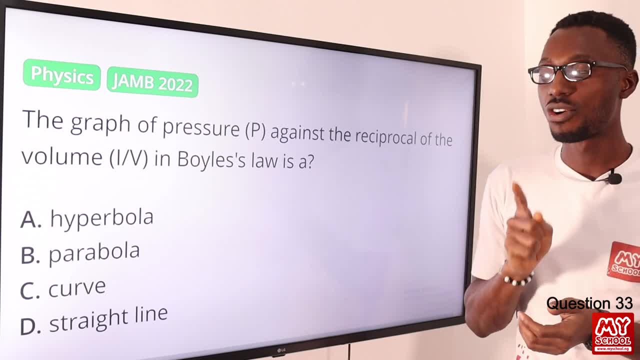 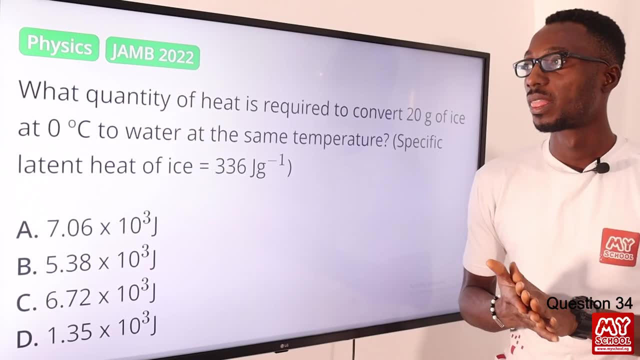 Is a straight line curve passing through the origin. all right, So take note of that. So the correct option is option D for a straight line Question 34.. What quantity of heat is required to convert 20 gram of ice at zero degrees Celsius to water? 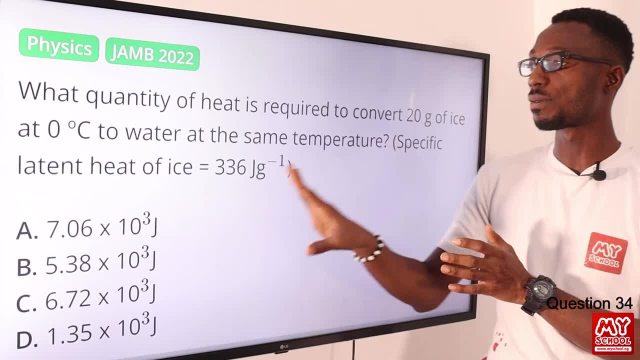 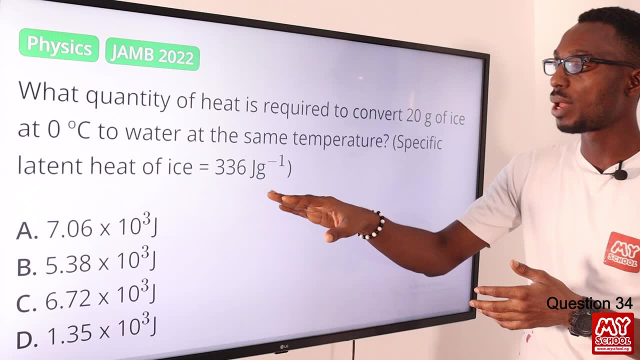 at the same temperature. So, given that specific latent heat of ice is 336 joules per gram, all right, So take note of the units being used. So right here we have joules per gram, not joules per kilogram, And right here I also have in gram, not in kilogram. So there's no need. 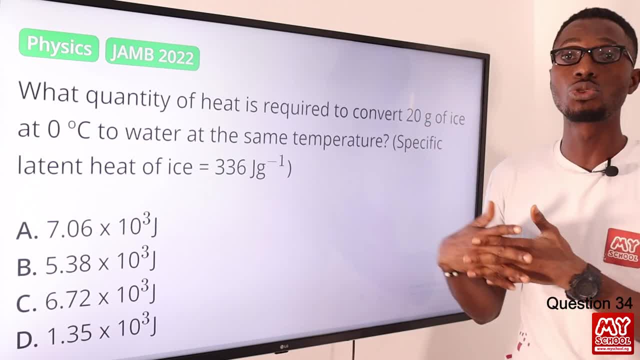 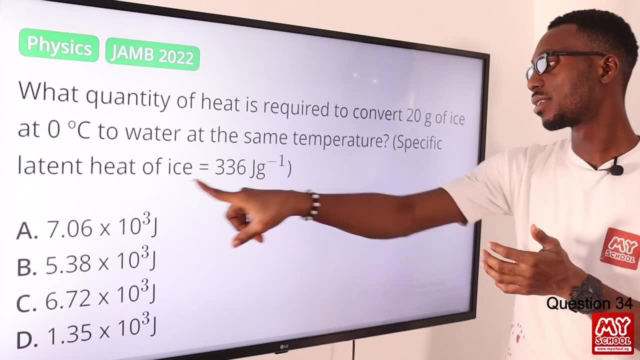 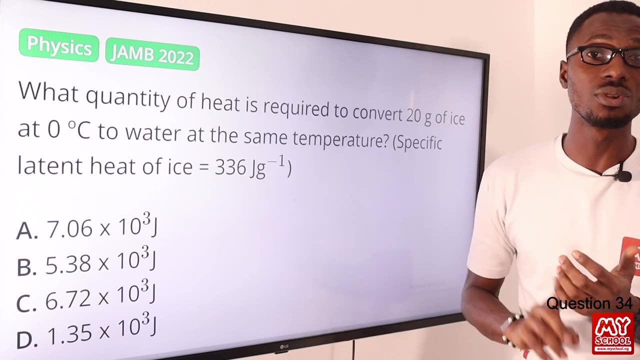 for conversion. So basically, if you record a rapport between the heat change or the quantity of the mass times, the- this times specific latent heat, right. So basically you just do 20 times 336. It's going to give me 6,720.. So if I bring it to standard form I will have 6.72 times 10 to the. 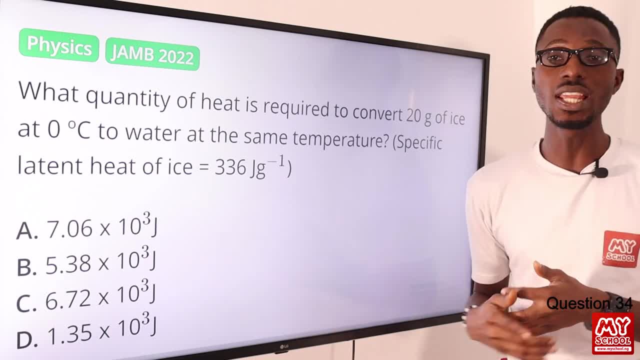 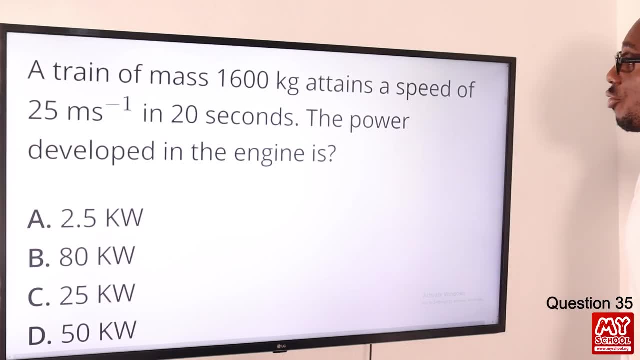 power 3 joules. You know it is measured in joules, So the correct option is option C 35.. A train of mass 1,600 kg attains a speed of 25 meters per second in 20 seconds. 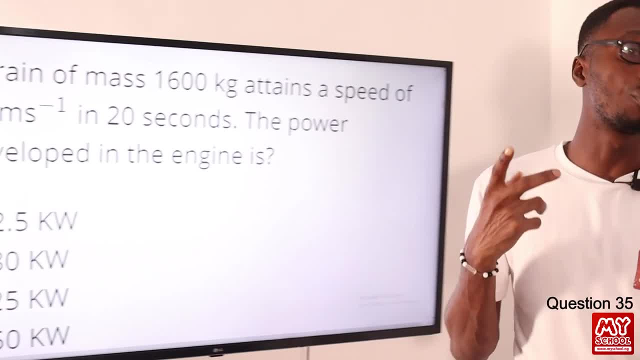 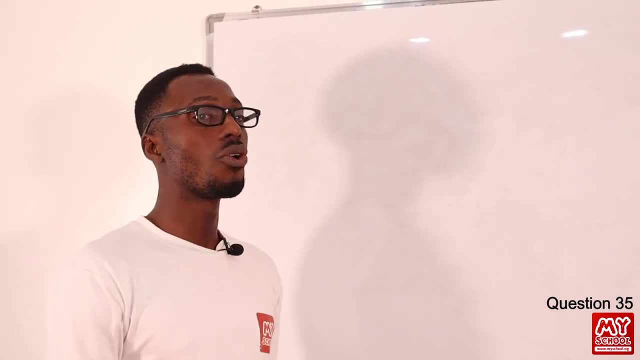 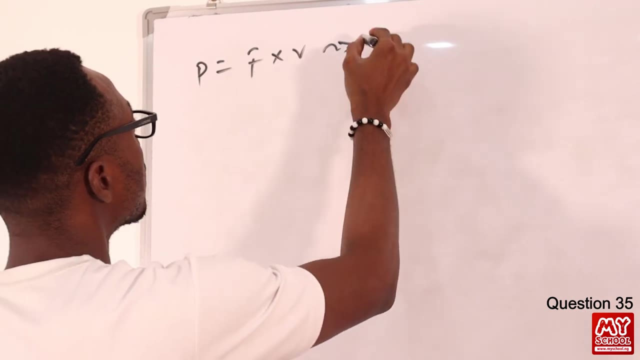 The power developed in the engine is what? So you just have to recall the proper formula, right? So we know that power is actually worked on over time. taking, Or you can also take, power, you know, equals your force times velocity. So right here we record our force is actually. 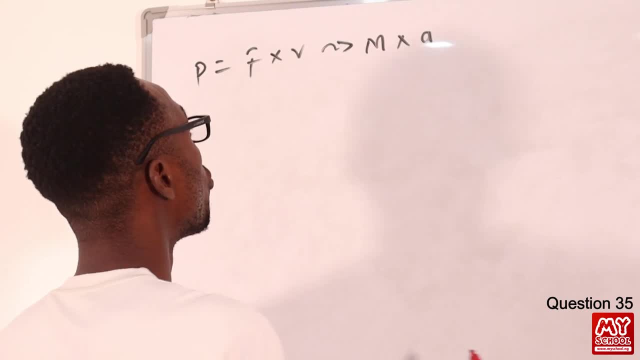 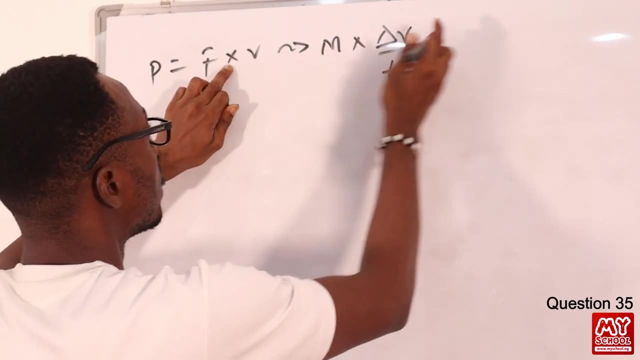 mass times, acceleration, okay, And we know that acceleration is actually changing velocity, you know, over time taking. So already we have a V standing here, Isn't it? So when we multiply it through, so we just have M right, We have V times V. 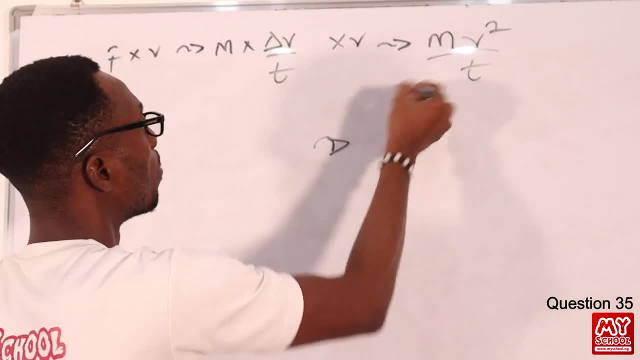 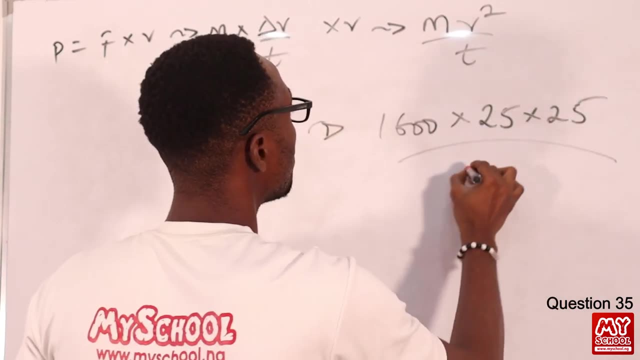 that is V squared over T. So just impute your formula. The mass is 1,600.. Then we have V squared, that is 25 times 25, right Over the time taking, that is 20 seconds. So when I divide this, 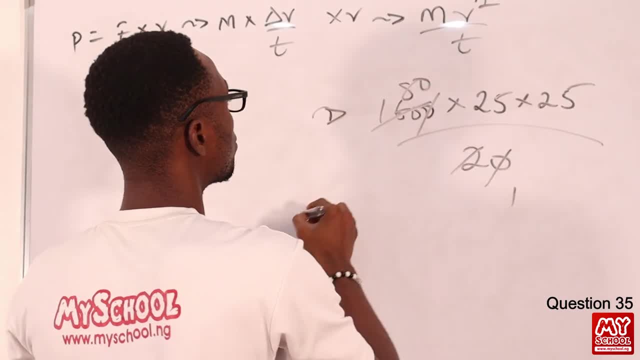 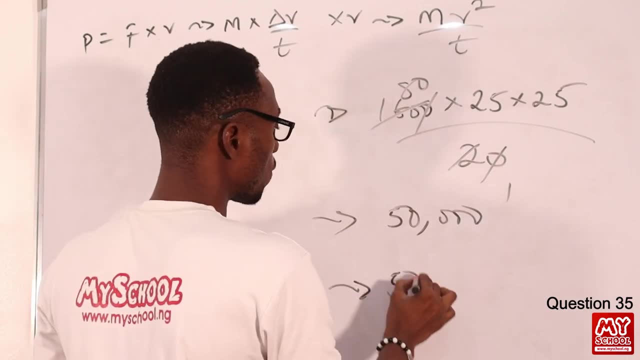 I have this here, I have 80.. When we multiply it through, basically we should have 50,000,. okay, So 50,000,. or if you want to convert kilowatts, you know, for power, it can be 50 kilowatts. Kilowatt kilo is 8,000.. So 1,000. 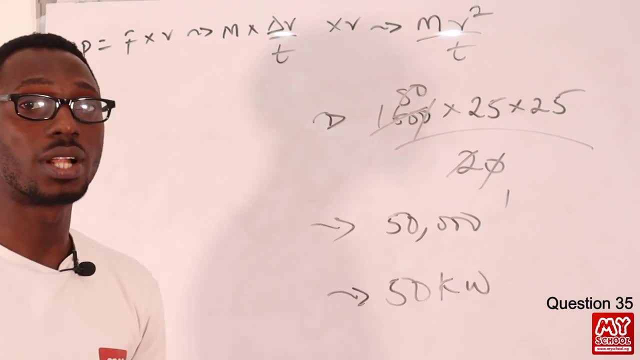 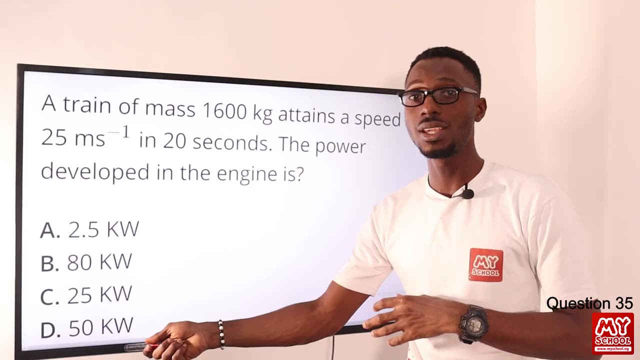 times 50, that is 50,000 watts or 50 kilowatts. So that's the correct value. So let's go back to the screen to secure the correct option. So we have that. Option D is the right option. 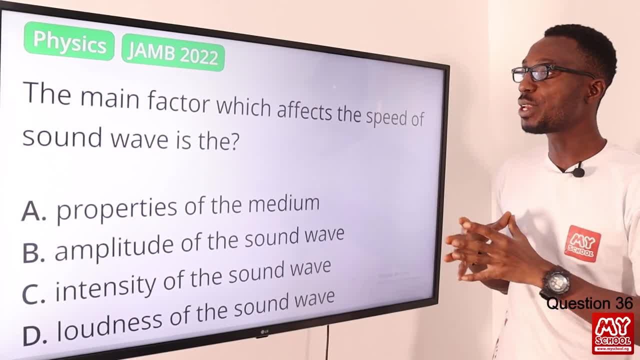 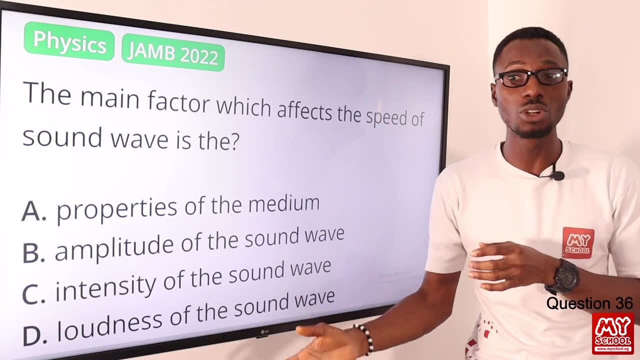 Number 36.. The main factor which affects the speed of sound wave is the water. They are the properties of the medium. all right, So first we want to consider what is the temperature that we are talking about. You know, temperature actually influences the speed of sound wave, not the salt. 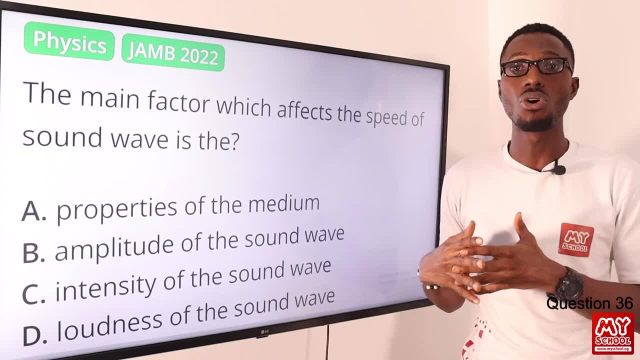 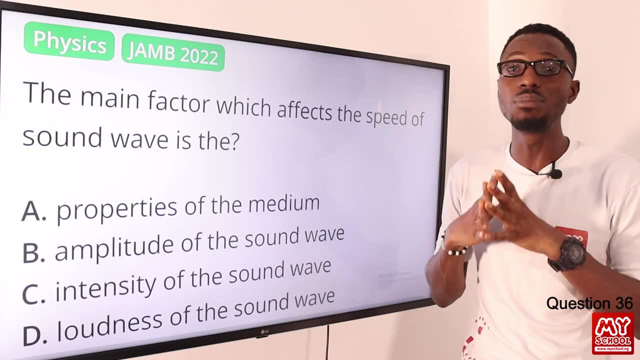 of the sound wave As well. you want to consider. you know other properties like the elasticity of the medium. you know the density of the medium. So basically, the properties of the medium is very essential. You know the property of the medium is very essential. you know, to the 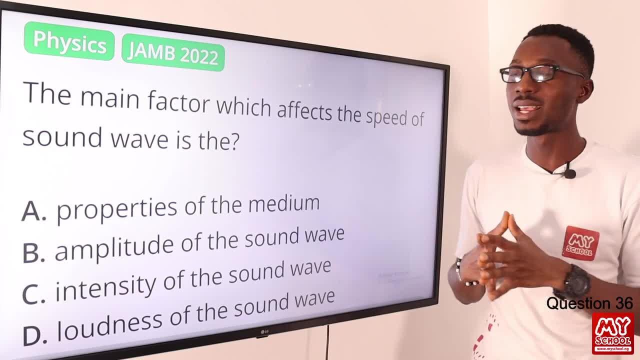 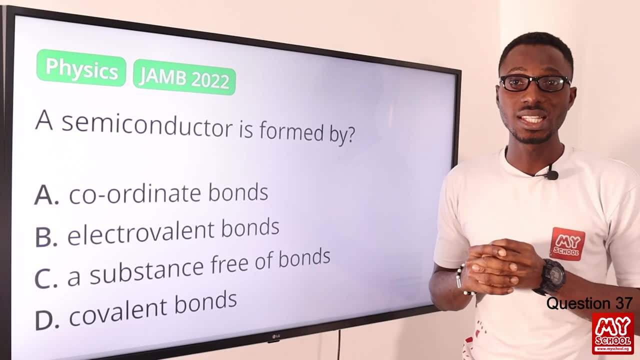 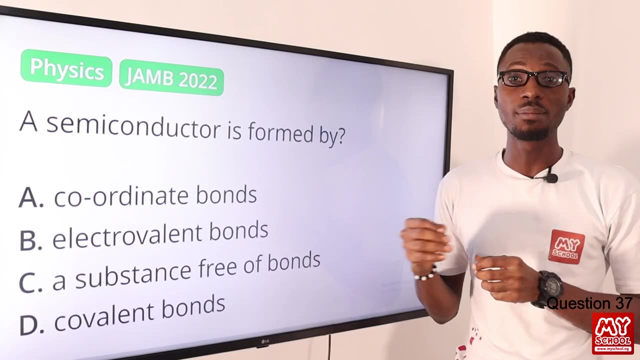 if, as well you know regarding the effect or how it affects the speed of sound wave. So the correct option is option A: The properties of the medium. Question 37.. A semiconductor is formed by what? By covalent bonds. You know you want to look at typical examples, like your silicon, like your germanium. 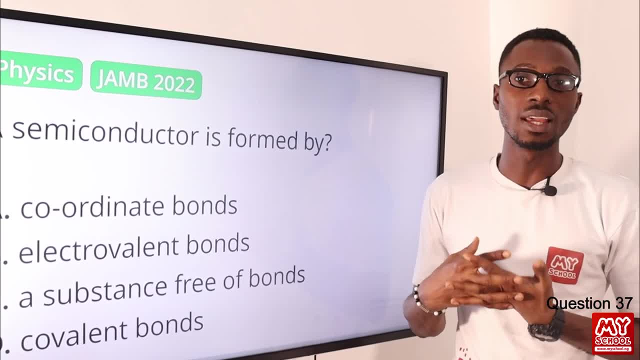 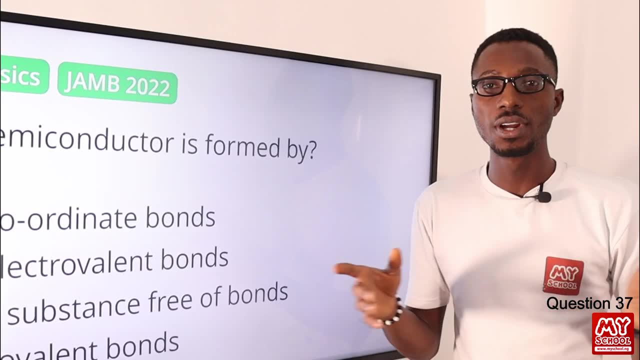 You know you find these in group 4 of the periodic table And even though the presence of a 4-valence electron, you know, these electrons are not really free to move like that. So basically you want to know that semiconductors, they are formed by the properties of the medium. 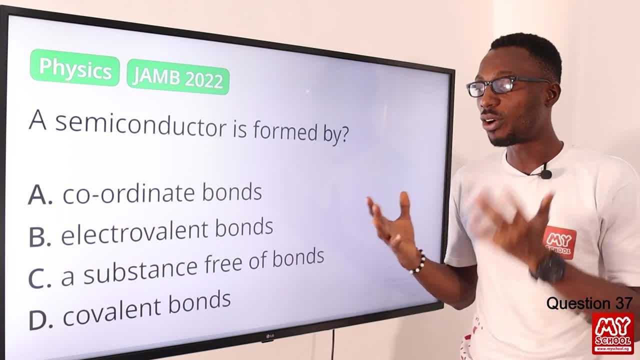 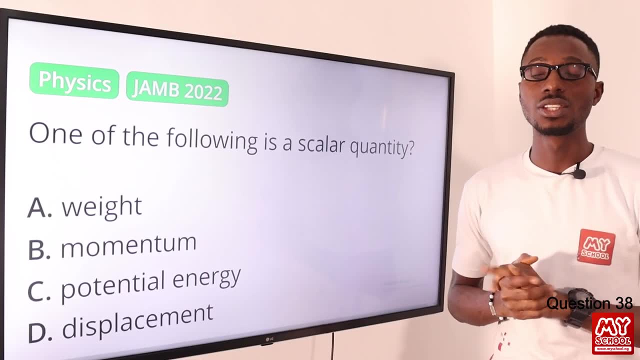 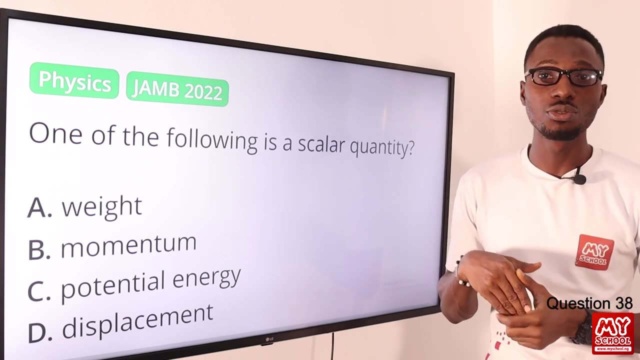 by this the covalent bond. so the correct option is option d for covalent bonds. 38. one of the following is a scalar quantity. so while we are looking at some scalar quantity, we are talking about magnitude but no direction. so, vector quantity, we have magnitude and we have direction. 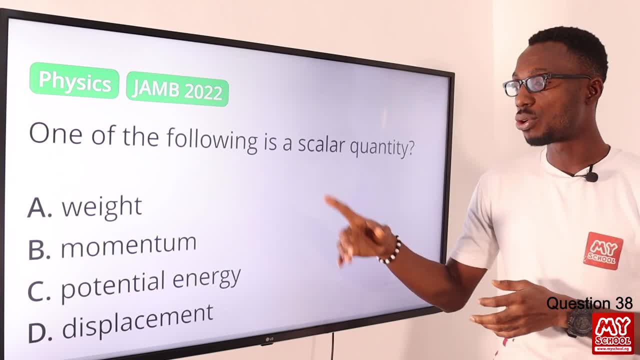 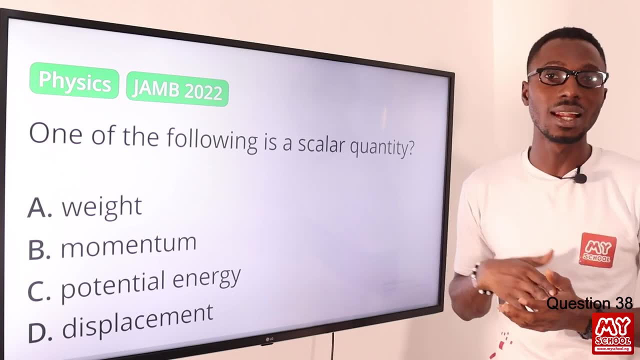 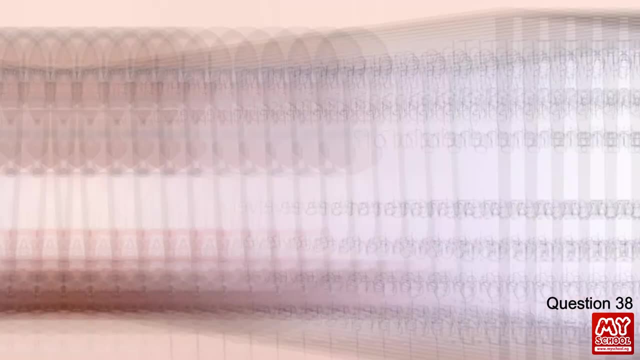 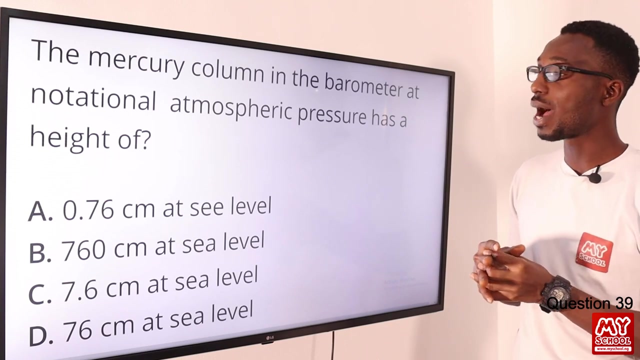 so examples include your weight, your momentum, your displacement and what have you? so energy generally. you know we take energy as a scalar quantity. because it is so, the correct option here is option c for potential energy. question 39: the mercury column in the barometer at notational atmospheric pressure has a height of what? so this is just a basic fact, you know we. 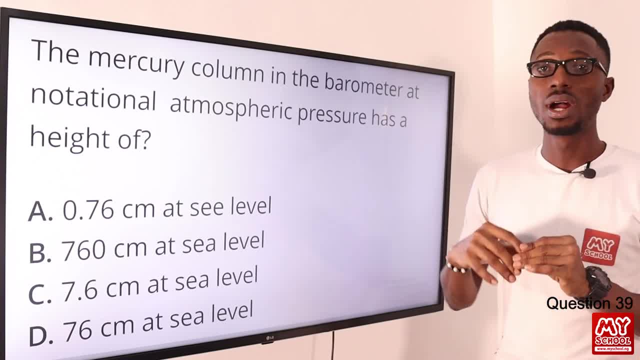 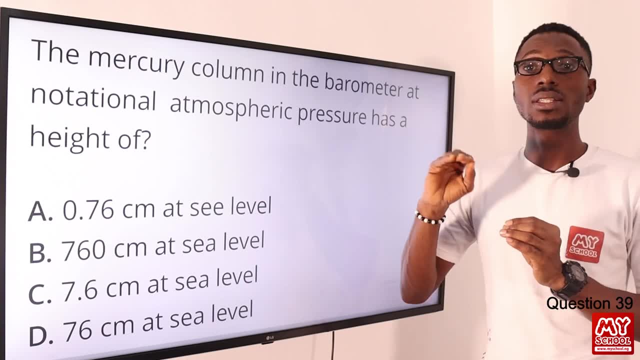 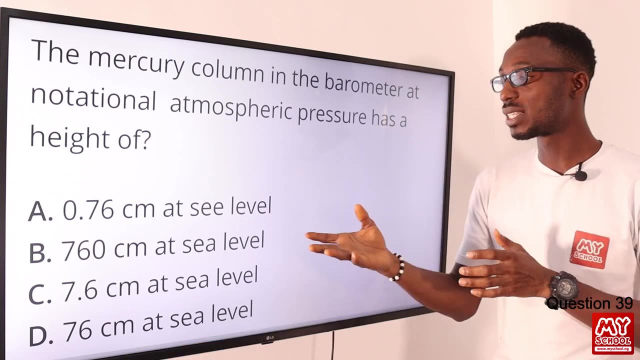 are talking about a reference point, all right, so that should be 76 centimeter at sea level. so some presentation can tell you 76 um 7, 60 millimeter, right so? but because we are using centimeter right there, so if you convert, of course you should have 76 centimeter at sea level. so this: 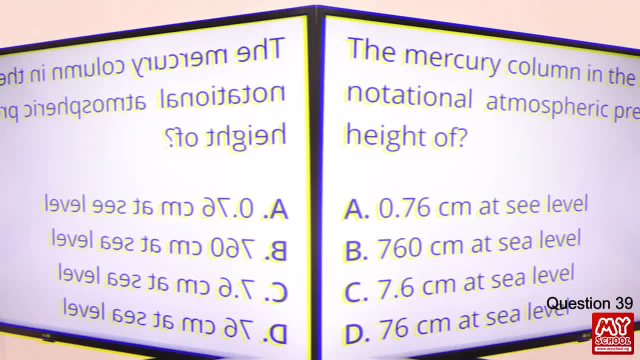 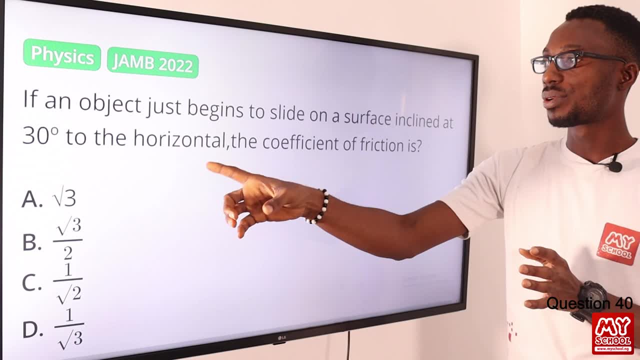 is the correct reference point. so option d is the right option. question number 40: and home jets just begins to slide on the surface, inclined at 30 degrees to the horizontal. so the coefficient of friction is what? so you just need to record the formula: the coefficient of static friction.